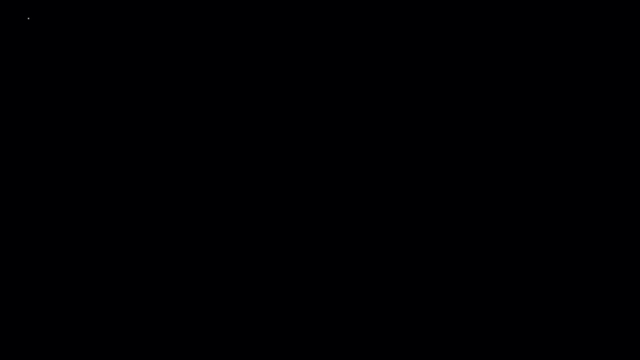 Let's talk about limits at infinity. What is the limit, as x approaches infinity, of 1 over x? What's the answer? Well, let's start plugging in large numbers. Whenever the denominator is large, you're going to get a small value. If the denominator has a small value, you get a large value. 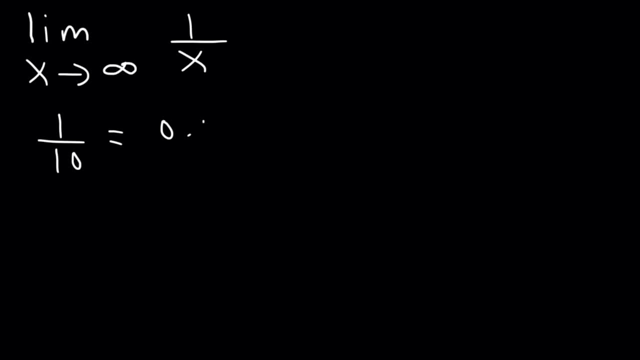 So, for example, 1 divided by 10 is 0.1.. 1 divided by 100 is 0.01.. And 1 divided by 1000 is 0.001.. Therefore, we can say that 1 over infinity, which is a very, very large number, is going to be about 0.. 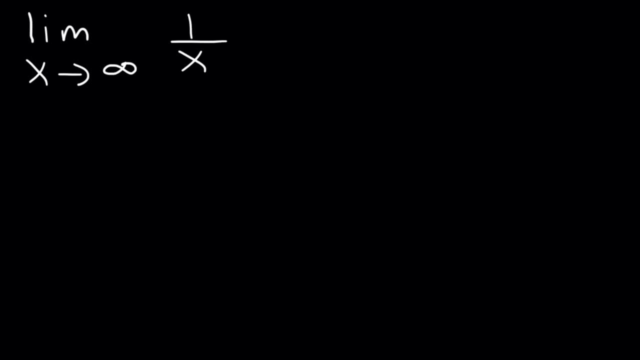 So the limit, as x approaches infinity, of 1 over x is therefore equal to 0.. Now what about the limit as x approaches negative infinity? 1 divided by negative infinity will still be 0.. If you divide 1 by negative 0.1, I mean by negative 10, rather, this would be negative 0.1.. 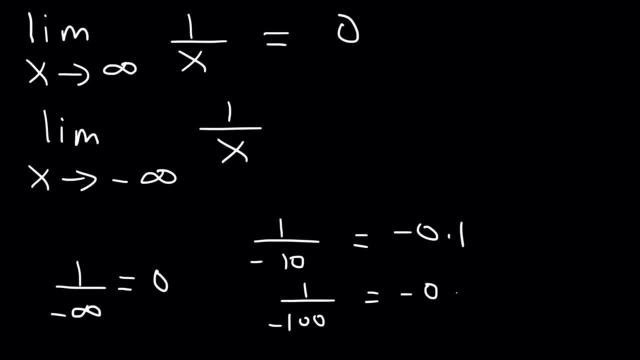 If you divide 1 by negative 100, you get negative 0.001.. I mean negative 0.01.. And if you divide it by negative 1000, you get negative 0.001.. It's still approaching 0, just from the left side. 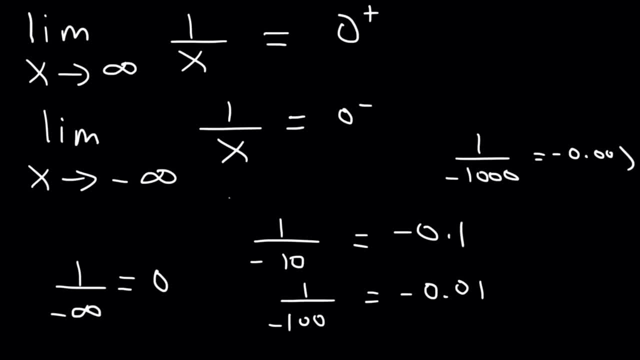 So this is 0. from the right side, This is equal to 0. from the left side, which you could just say it's equal to 0.. Now let's graph this function. The graph of 1 over x looks like this: 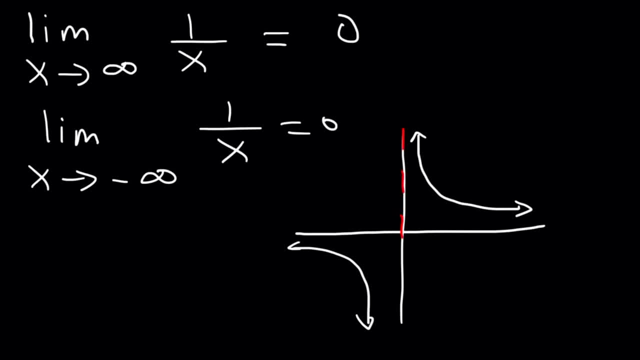 It has a vertical asymptote at x equals 0.. And it has a horizontal asymptote At y equals 0.. So, as you can see, as x approaches positive infinity, you're going to get the horizontal asymptote, which is y is equal to 0.. 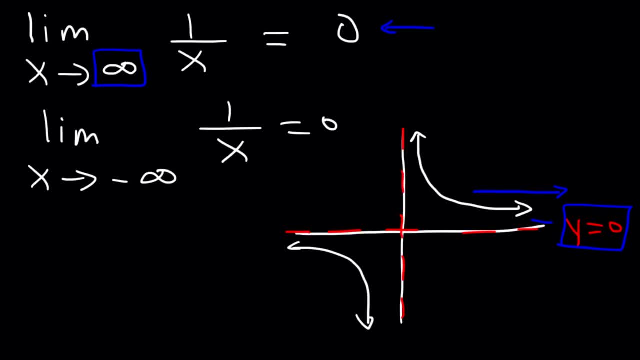 As we follow the curve all the way to the right, it's going to get closer and closer to 0.. This will also give you the horizontal asymptote on the left side, which is also y, equals 0.. To get the vertical asymptote, as x approaches 0 from the right side. 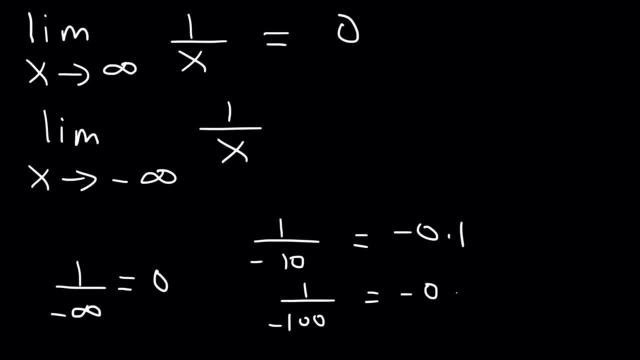 If you divide 1 by negative 100, you get negative 0.001.. I mean negative 0.01.. And if you divide it by negative 1000, you get negative 0.001.. It's still approaching 0, just from the left side. 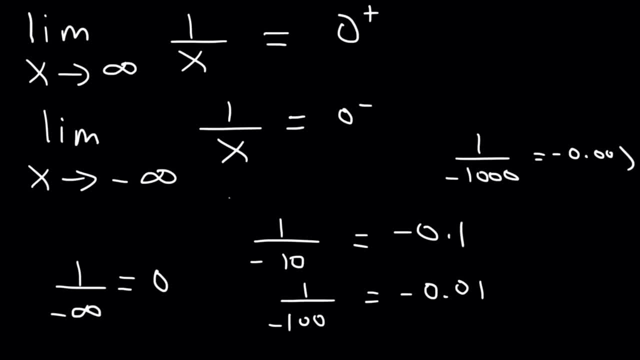 So this is 0. from the right side, This is equal to 0. from the left side, which you could just say it's equal to 0.. Now let's graph this function. The graph of 1 over x looks like this: 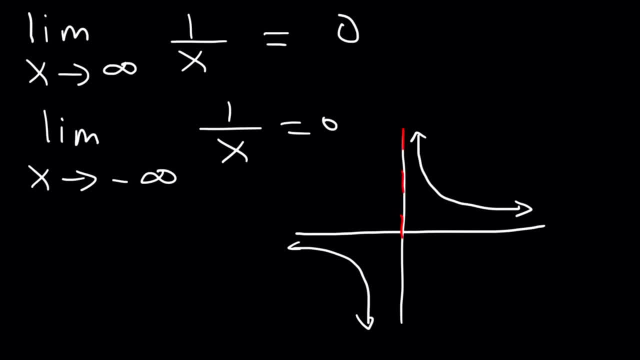 It has a vertical asymptote at x equals 0.. And it has a horizontal asymptote At y equals 0.. So, as you can see, as x approaches positive infinity, you're going to get the horizontal asymptote, which is y is equal to 0.. 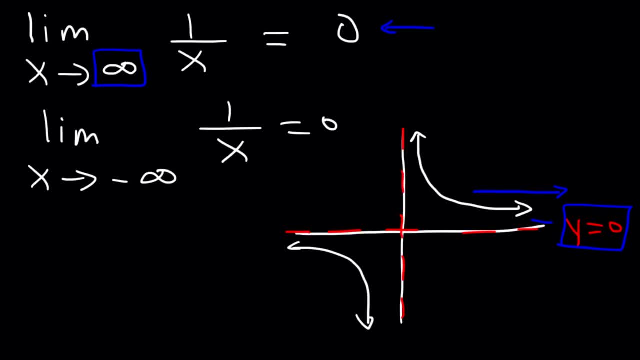 As we follow the curve all the way to the right, it's going to get closer and closer to 0.. This will also give you the horizontal asymptote on the left side, which is also y, equals 0.. To get the vertical asymptote, as x approaches 0 from the right side. 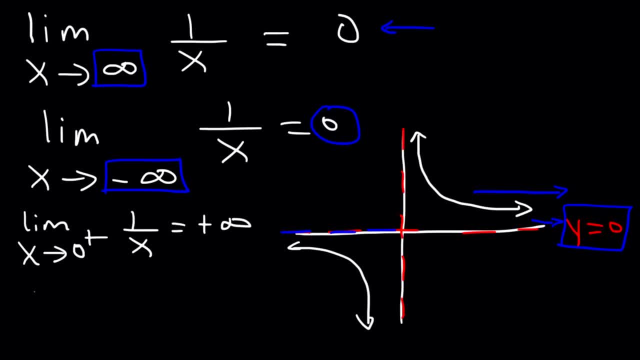 this will give us positive infinity. So that tells you that 0 is a vertical asymptote. If you approach 0 from the left side, you're going to get negative infinity. It's going down, So the x value that leads to a y value of infinity. 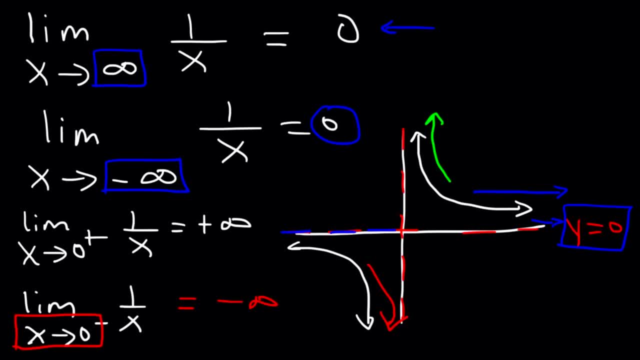 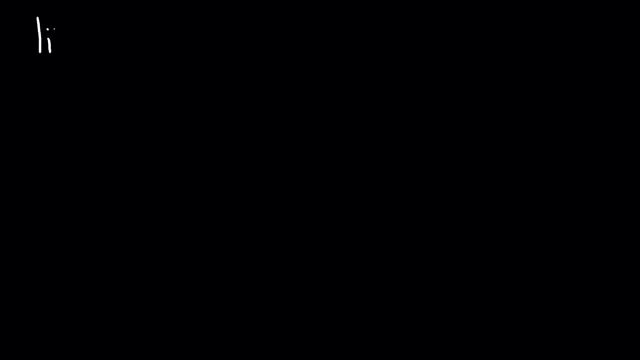 that's going to be the vertical asymptote. When x approaches infinity, the y value corresponds to negative infinity. So that's going to be the vertical asymptote. So the horizontal asymptote. Let's try another problem. What is the limit, as x approaches infinity, of 1 over x squared? 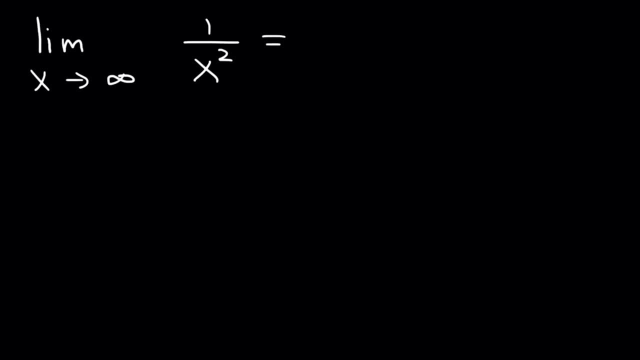 Well, here we have another bottom-heavy function. And if we plug in a large number, let's say like 100.. 100 squared is 10,000.. And 1 divided by 10,000 is still a very small number: 0.0001.. 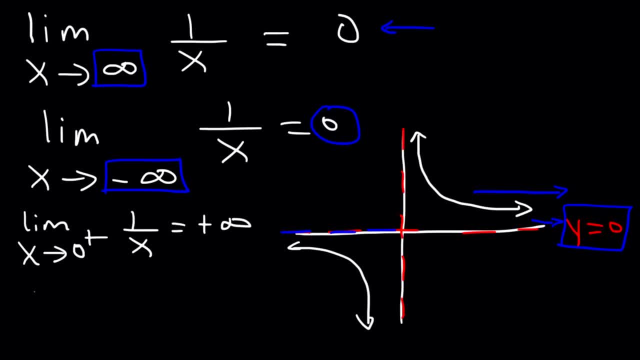 this will give us positive infinity. So that tells you that 0 is a vertical asymptote. If you approach 0 from the left side, you're going to get negative infinity. It's going down, So the x value that leads to a y value of infinity. 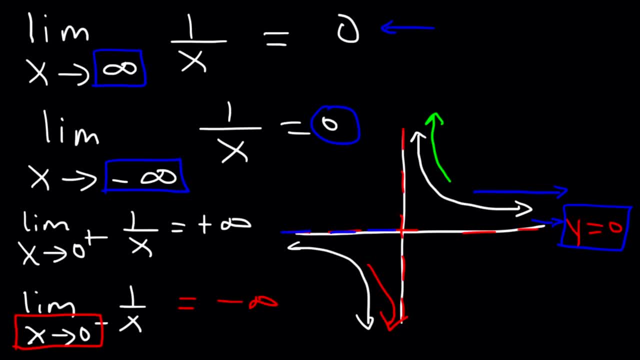 that's going to be the vertical asymptote. When x approaches infinity, the y value corresponds to negative infinity. So when x approaches infinity, the y value corresponds to negative infinity. So the horizontal asymptote. Let's try another problem. 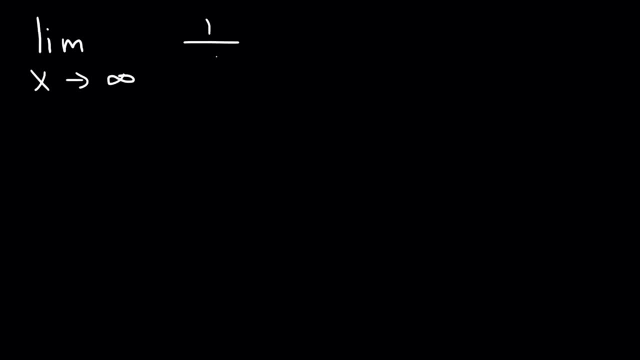 What is the limit, as x approaches infinity, of 1 over x squared? Well, here we have another bottom-heavy function, And if we plug in a large number, let's say like 100.. 100 squared is 10,000.. And 1 divided by 10,000 is still a very small number, 0.0001.. 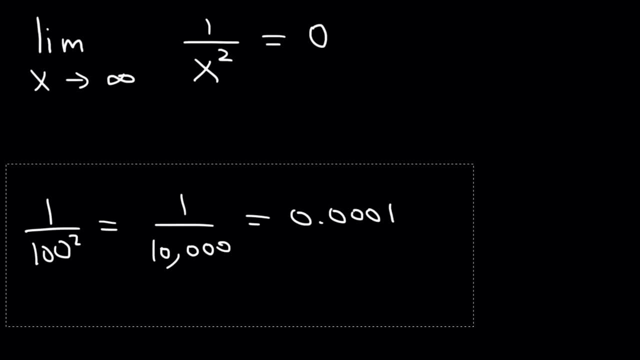 So we can say this is going to approach 0. Any time you have 1 divided by infinity, it's always going to equal 0. So here's a general theorem: The limit as x approaches infinity of some function: 1 over x to the r. 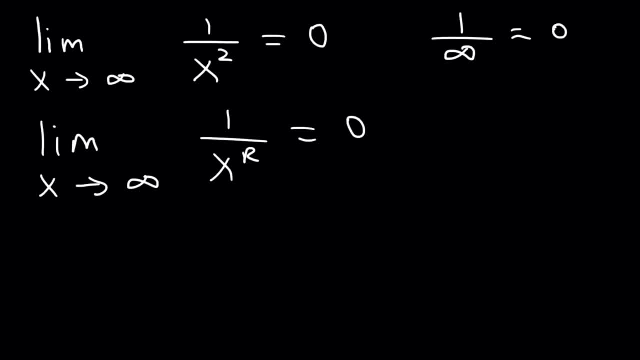 will always be equal to 0. So that's something that you may want to keep in mind. What is the limit, as x approaches infinity, of 8 divided by 3x plus 0?? It's 4.. So what process can we use to figure this out? 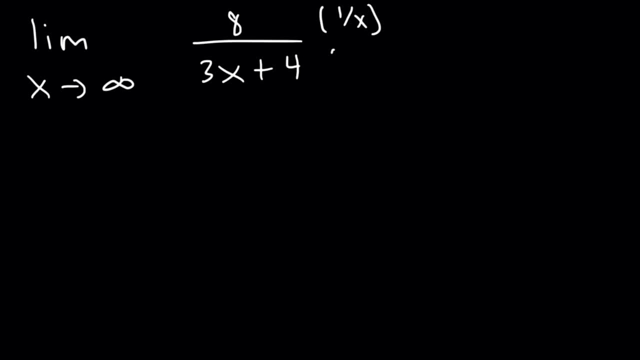 What we need to do is multiply the top and the bottom by 1 over x, And so this is going to be equal to 8 divided by x. And then, on the bottom, we're going to distribute 3x times. 1 over x is 3.. 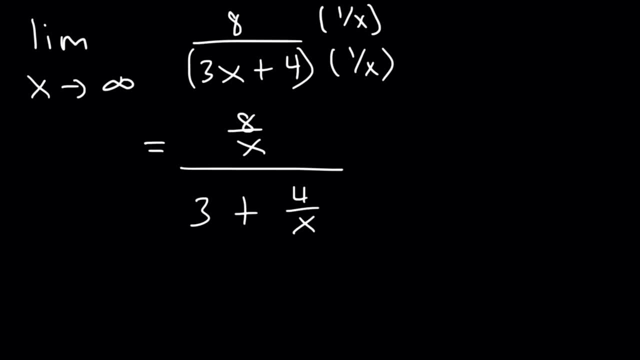 And 4 times 1 over x is 4 over x. So now we can apply the limit as x approaches infinity For every term in this fraction. So recall any time you have, let's say, a fraction like 1 over x. 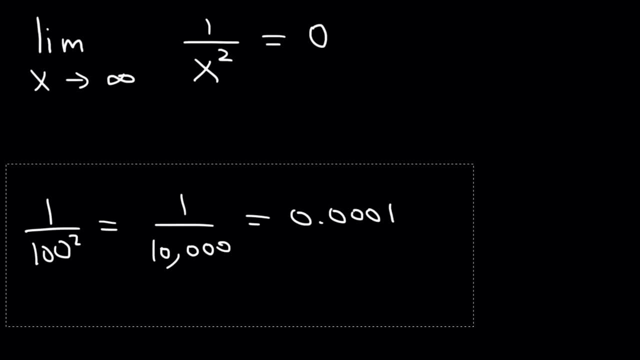 So we can say this is going to approach 0. Any time you have 1 divided by infinity, it's always going to equal 0. So here's a general theorem: The limit as x approaches infinity of some function: 1 over x to the r. 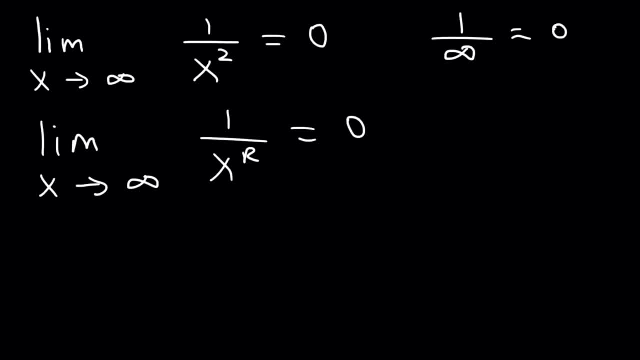 will always be equal to 0. So that's something that you may want to keep in mind. What is the limit, as x approaches infinity, of 8 divided by 3x plus 0?? It's 4.. So what process can we use to figure this out? 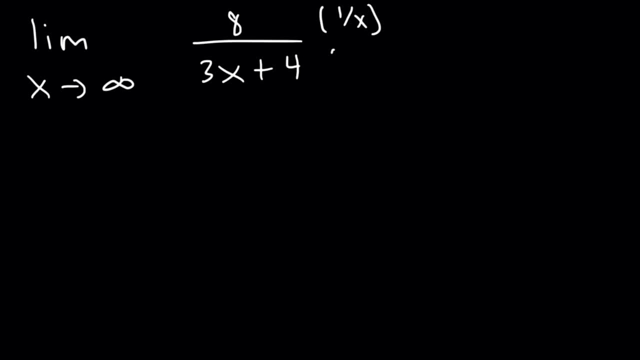 What we need to do is multiply the top and the bottom by 1 over x, And so this is going to be equal to 8 divided by x. And then, on the bottom, we're going to distribute 3x times. 1 over x is 3.. 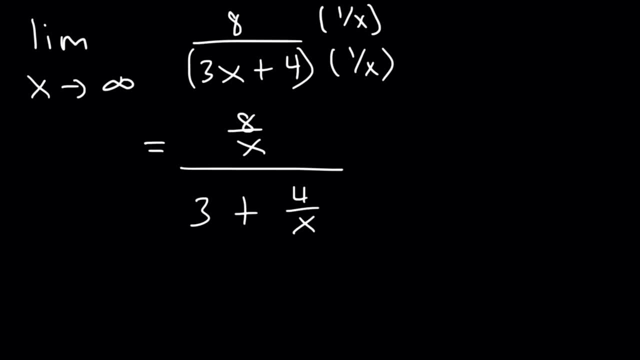 And 4 times 1 over x is 4 over x. So now we can apply the limit as x approaches infinity For every term in this fraction. So recall any time you have, let's say, a fraction like 1 over x. 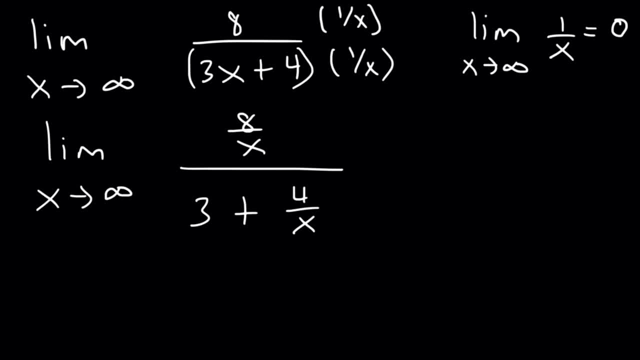 that's going to turn into 0.. The limit as x approaches infinity for 1 over x is 0. So we can rewrite this as the limit. Well, this is going to be. let's separate the 8 from 1 over x. 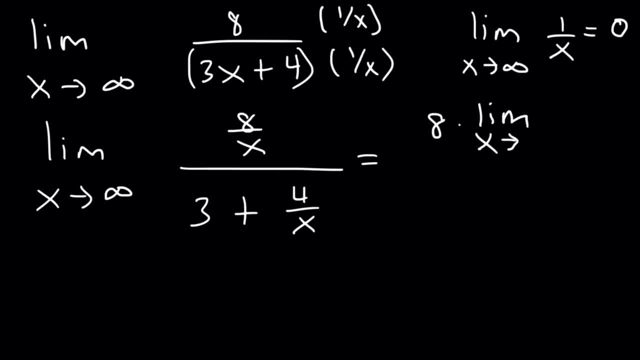 So it's 8 times the limit as x approaches infinity 1 over x over 3, plus 4 times the limit as x approaches infinity 1 over x, If you want to show every step. So we know this portion is equal to 0.. 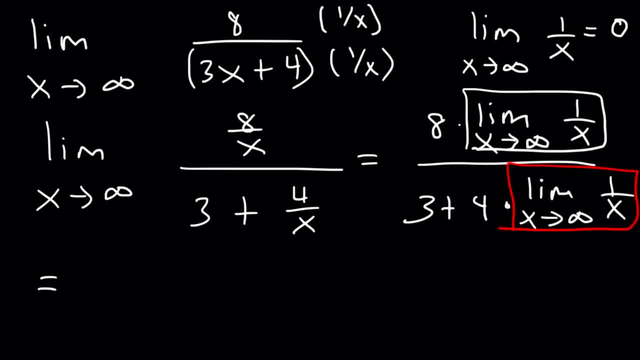 And the same is true for this part. So it's going to be 8 times 0 divided by 3 plus 4 times 0. So this is 0 over 3 plus 0, which is 0 over 3.. 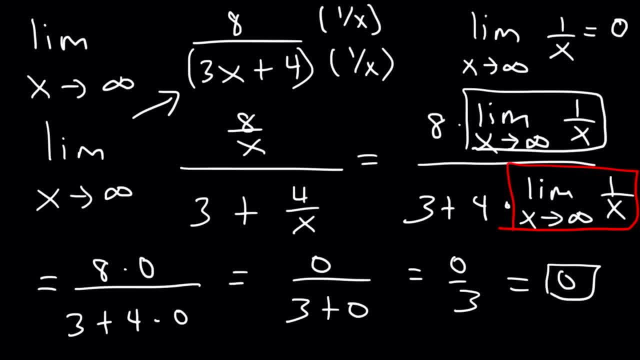 Basically, the whole thing is 0. So any time the function is bottom heavy, notice that the degree of the denominator is greater than that of the numerator. Any time it's bottom heavy, it's going to equal 0.. Now let's work on something else. 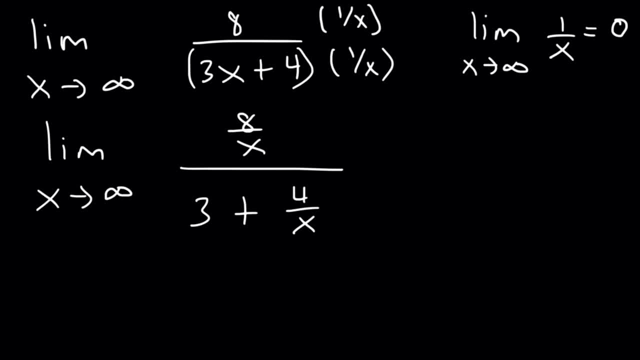 that's going to turn into 0.. The limit as x approaches infinity for 1 over x is 0. So we can rewrite this as the limit. Well, this is going to be. let's separate the 8 from 1 over x. 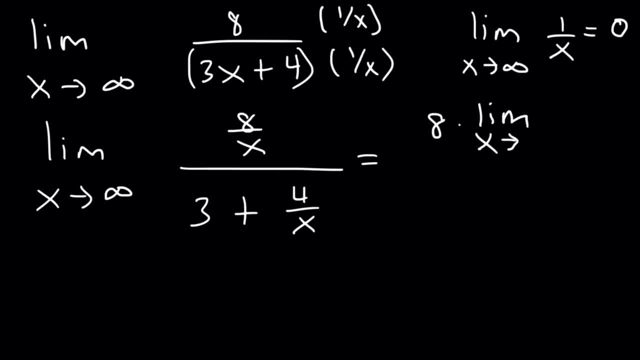 So it's 8 times the limit as x approaches infinity 1 over x over 3, plus 4 times the limit as x approaches infinity 1 over x, If you want to show every step. So we know this portion is equal to 0.. 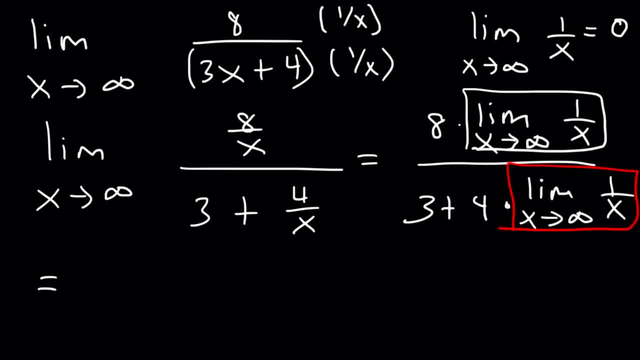 And the same is true for this part. So it's going to be 8 times 0 divided by 3 plus 4 times 0. So this is 0 over 3 plus 0, which is 0 over 3.. 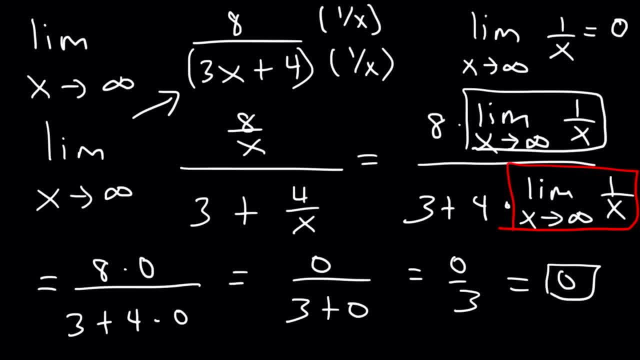 Basically, the whole thing is 0. So any time the function is bottom heavy, notice that the degree of the denominator is greater than that of the numerator. Any time it's bottom heavy, it's going to equal 0.. Now let's work on something else. 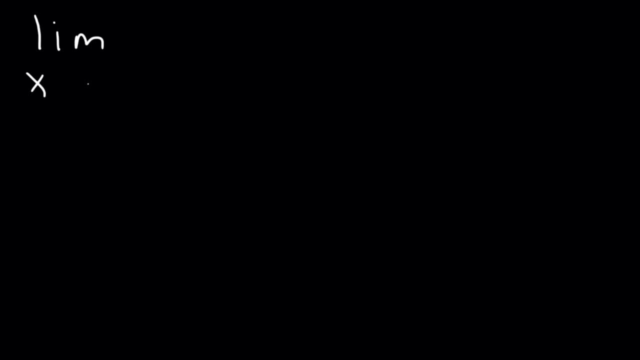 What is the limit, as x approaches infinity, of 8x minus 5 divided by 2x plus 3?? So what is the answer in this case? Now notice that the degree of the numerator is the same as that of the denominator. 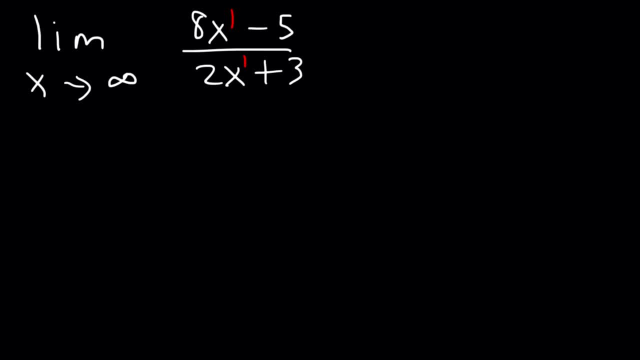 They're both to the first power, So they're in the first degree. Whenever the degree of the numerator and the denominator is the same, you can simply divide the coefficients. So 8 divided by 2 is 4.. Therefore, this is going to equal 4.. 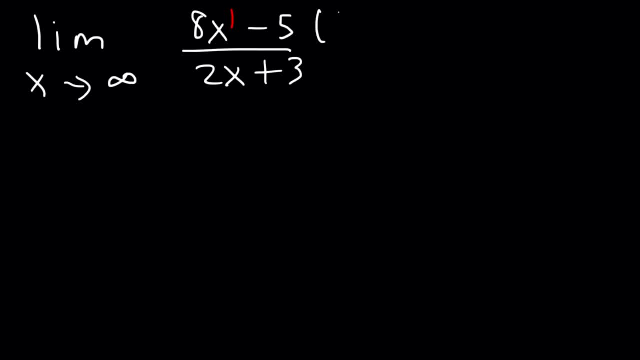 Now let's prove it, Let's show our work. So I'm going to multiply the top and the bottom by 1 over x. So I'm going to multiply the top and the bottom by 1 over x. So I'm going to multiply the top and the bottom by 1 over x. 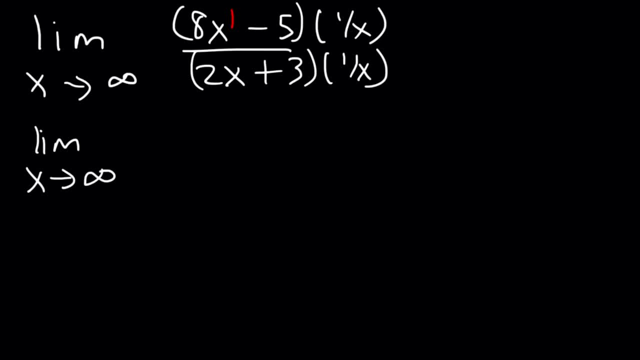 So, therefore, this is going to be the limit as x approaches infinity. 8x times 1 over x is simply 8.. And then we're going to have 5 times 1 over x, which is 5 over x. 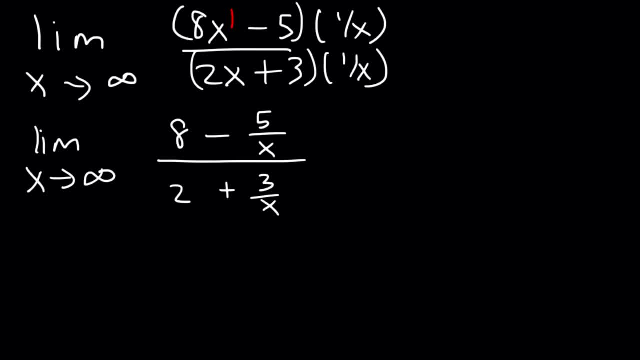 And then this is going to be 2 plus 3 over x. The limit, as x approaches infinity, of 5 over x is going to equal 0.. If you want to write it out separately, you can write it out as 5 times the limit as x approaches infinity of 1 over x. 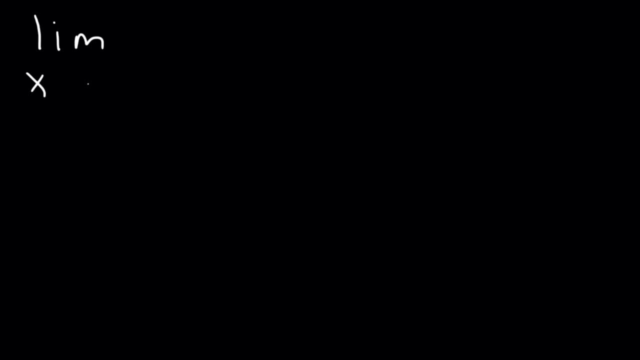 What is the limit, as x approaches infinity, of 8x minus 5 divided by 2x plus 3?? So what is the answer in this case? Now notice that the degree of the numerator is the same as that of the denominator. 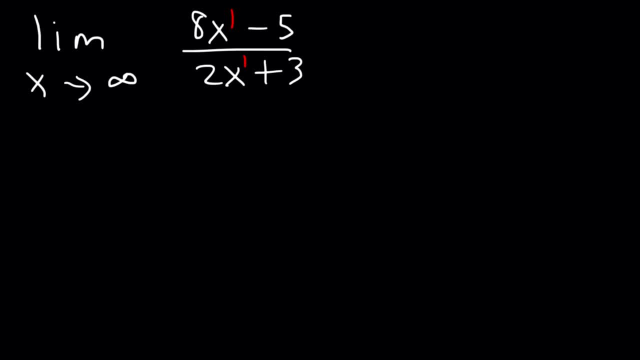 They're both to the first power, So they're in the first degree. Whenever the degree of the numerator and the denominator is the same, you can simply divide the coefficients. So 8 divided by 2 is 4.. Therefore, this is going to equal 4.. 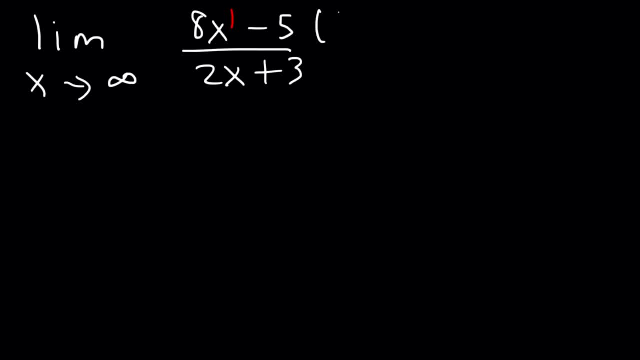 Now let's prove it, Let's show our work. So I'm going to multiply the top and the bottom by 1 over x. So I'm going to multiply the top and the bottom by 1 over x. So I'm going to multiply the top and the bottom by 1 over x. 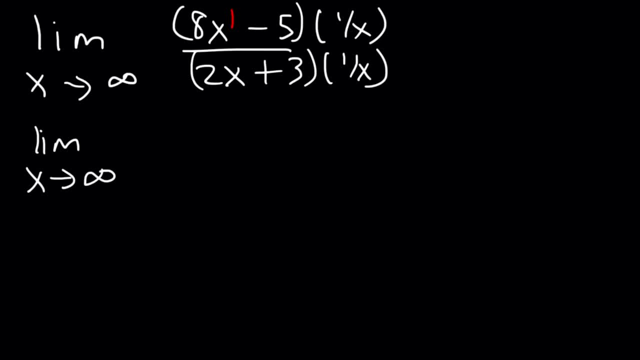 So, therefore, this is going to be the limit as x approaches infinity. 8x times 1 over x is simply 8.. And then we're going to have 5 times 1 over x, which is 5 over x. 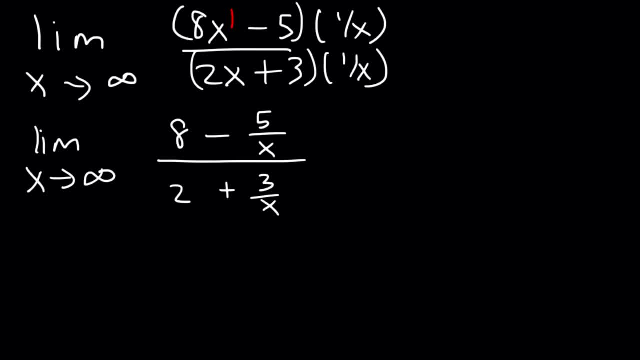 And then this is going to be 2 plus 3 over x. The limit, as x approaches infinity, of 5 over x is going to equal 0.. If you want to write it out separately, you can write it out as 5 times the limit as x approaches infinity of 1 over x. 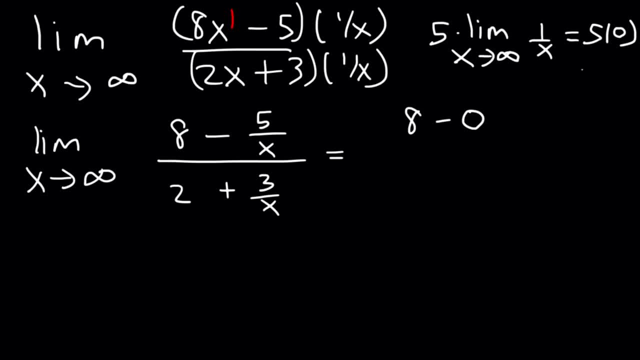 So that's 5 times 0, which in the end is going to be 0.. Now 3 over x, that's also going to change into 0. So 8 divided by 2 is 4.. So keep in mind, for those of you who want to write out every step, you can write it like this if you want to. 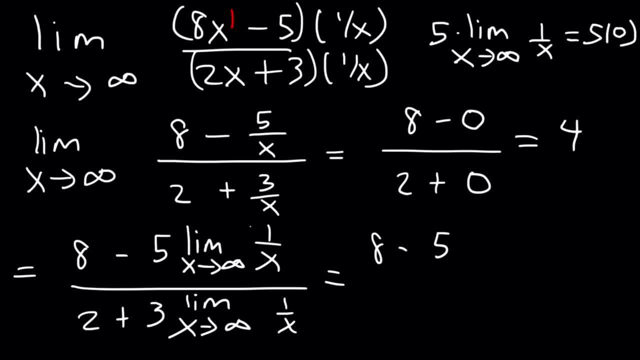 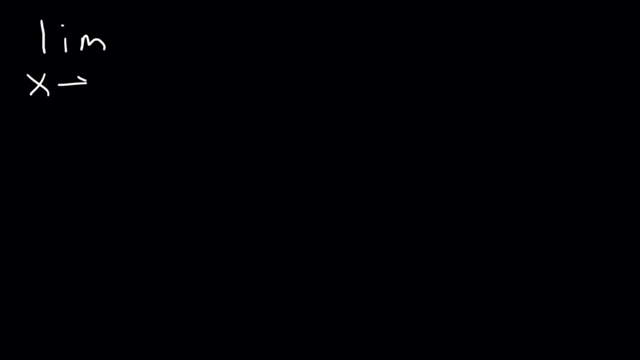 And then you can apply this, The formula: Since this is a rational function, it's going to equal 0. But in the end you're going to get the same answer: positive, 4.. What is the limit, as x approaches infinity, of 5 minus 7x cubed divided by 3x plus 5x cubed plus 9?? 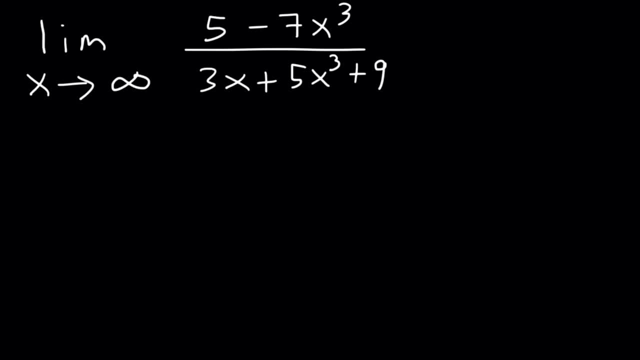 Go ahead and try this. So notice that the degree of the numerator is 3, and the degree of the denominator is 3.. That's the highest exponent on top and on the bottom. So you could say that as x becomes large, 5 is insignificant to 7x cubed. 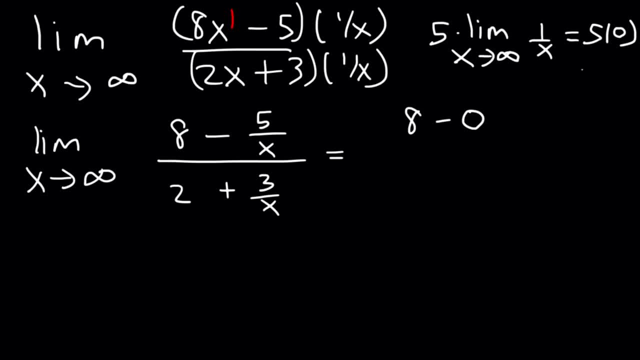 So that's 5 times 0, which in the end is going to be 0.. Now 3 over x, that's also going to change into 0. So 8 divided by 2 is 4.. So keep in mind, for those of you who want to write out every step, you can write it like this if you want to. 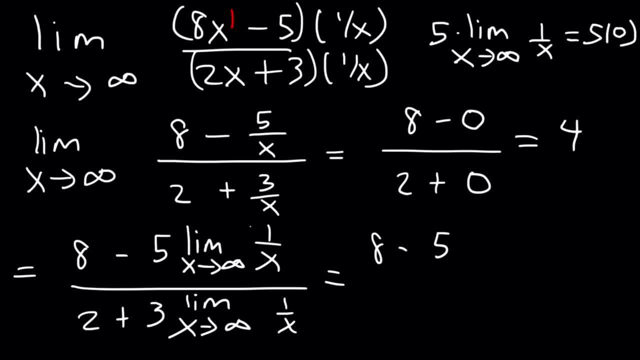 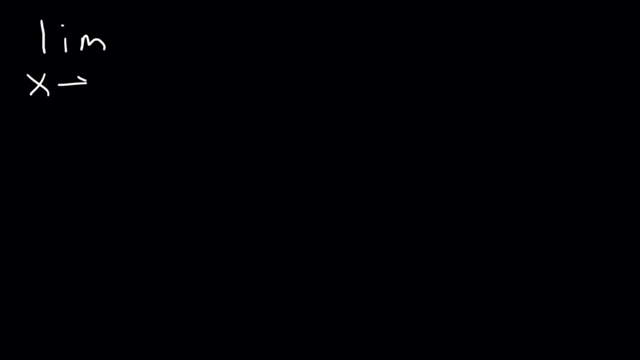 And then you can apply this, The formula: Since this is a rational function, it's going to equal 0. But in the end you're going to get the same answer: positive, 4.. What is the limit, as x approaches infinity, of 5 minus 7x cubed divided by 3x plus 5x cubed plus 9?? 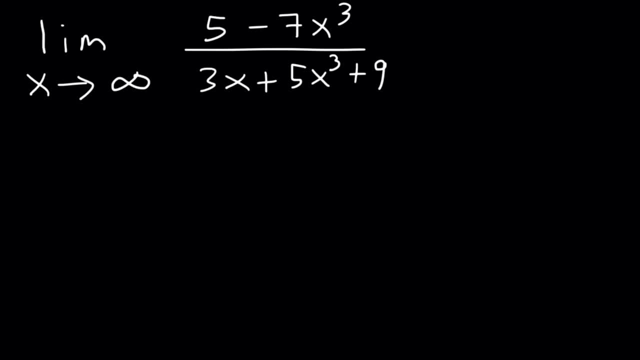 Go ahead and try this. So notice that the degree of the numerator is 3, and the degree of the denominator is 3.. That's the highest exponent on top and on the bottom. So you could say that as x becomes large, 5 is insignificant to 7x cubed. 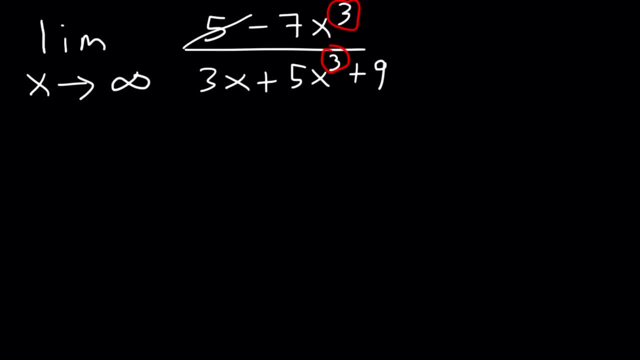 Because if you plug in 1,000 into x, 1,000 to the third is a billion times 7,, that's 7 billion. 5 is insignificant to that. So 3x and 9 are insignificant to 5x cubed. 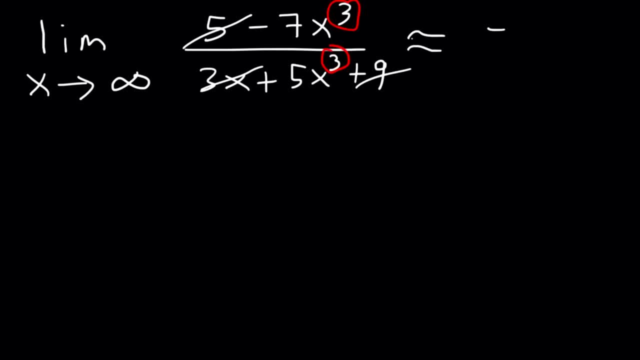 So this is approximately Equal to negative 7x cubed divided by 5x cubed, which the answer turns out to be negative 7 over 5.. But let's confirm it. So what we need to do is multiply the top and the bottom, this time by 1 over x cubed. 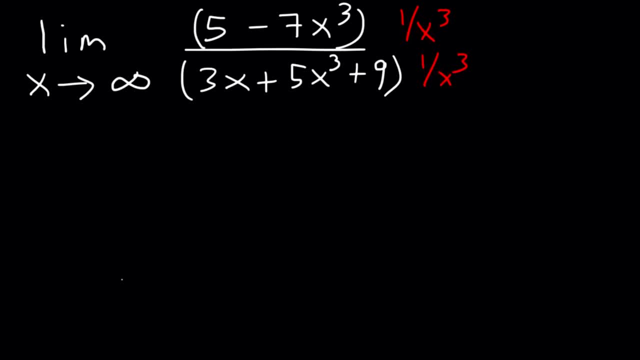 Since the highest degree is x cubed or 3.. So this is going to be the limit as x approaches infinity: 5 over x cubed, minus 7 divided by 3 over x squared, plus 5 plus 9 over x cubed. 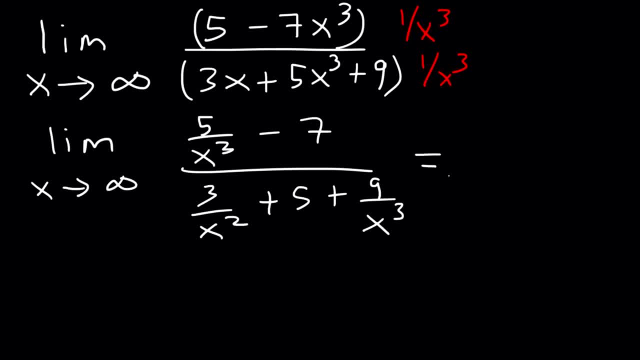 5 divided by infinity to the third power is going to be 0.. Anytime you have infinity in the bottom of a fraction, it's 0. So we're going to have 0 minus 7.. 3 over infinity squared, that's going to be 0, plus 5, plus 9 over infinity cubed, which is 0.. 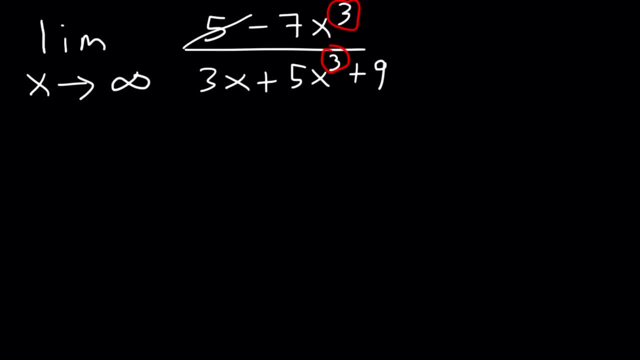 Because if you plug in 1,000 into x, 1,000 to the 3rd is a billion times 7, that's 7 billion. 5 is insignificant to that. So 3x and 9 are insignificant to 5x cubed. 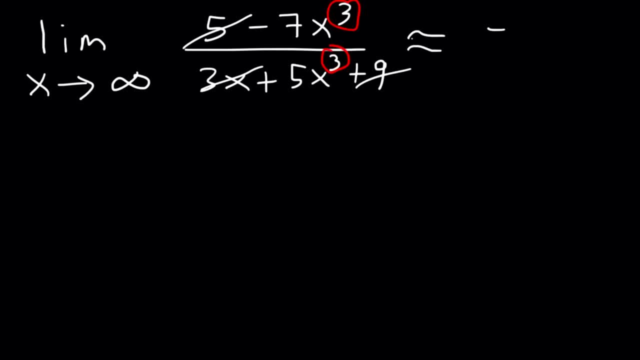 So this is approximately Equal to negative 7x cubed divided by 5x cubed, which the answer turns out to be negative 7 over 5.. But let's confirm it. So what we need to do is multiply the top and the bottom, this time by 1 over x cubed. 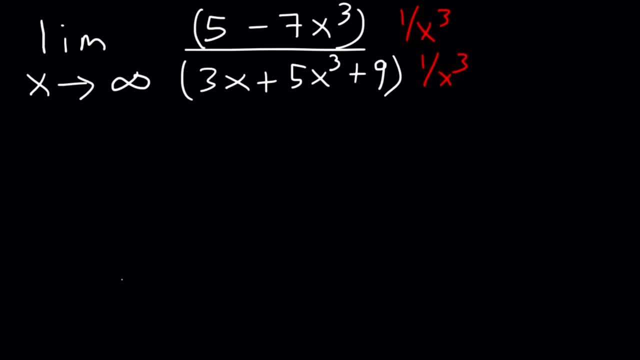 Since the highest degree is x cubed or 3.. So this is going to be the limit as x approaches infinity: 5 over x cubed, minus 7 divided by 3 over x squared, plus 5 plus 9 over x cubed. 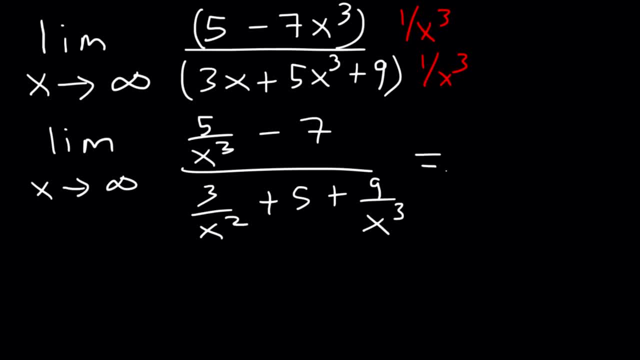 5 divided by infinity to the 3rd power is going to be 0.. Anytime you have infinity in the bottom of a fraction, it's 0. So we're going to have 0 minus 7.. 3 over infinity squared, that's going to be 0, plus 5, plus 9 over infinity cubed, which is 0.. 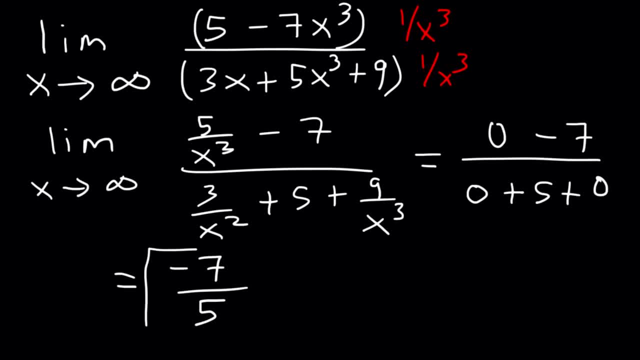 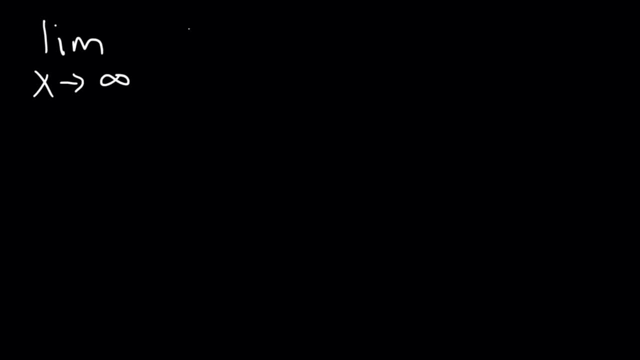 So in the end you get negative 7. Divided by 5.. What is the limit, as x approaches infinity, of the square root of 16x squared minus 8, divided by 2x minus 5?? Go ahead and try it. 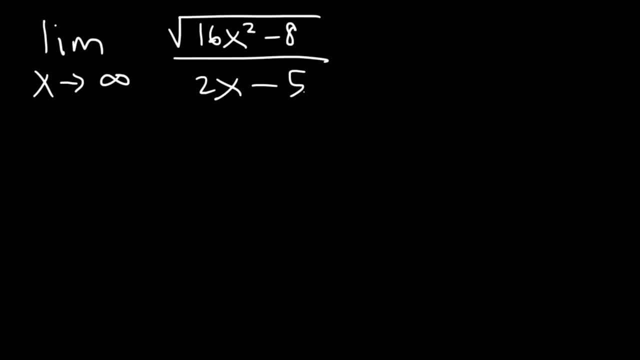 So when x is very large, only the most significant term will remain or will be important. 8 is insignificant and 5 is insignificant. So this expression: It becomes equal to the square root of 16x squared divided by 2x. 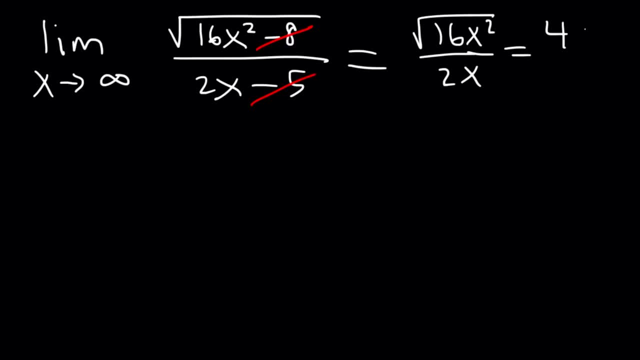 The square root of 16 is 4, and the square root of x squared is x, And 4x divided by 2x is 2.. So that's going to be the answer, But now let's confirm it with a step-by-step process. 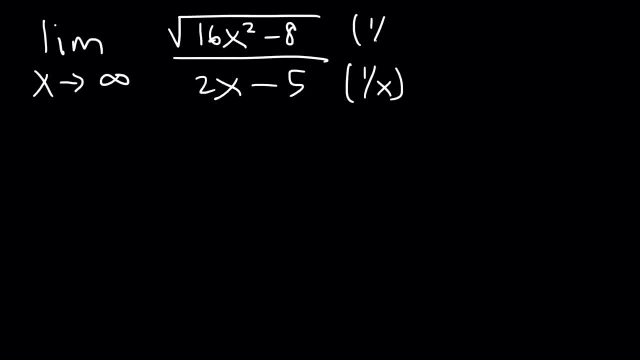 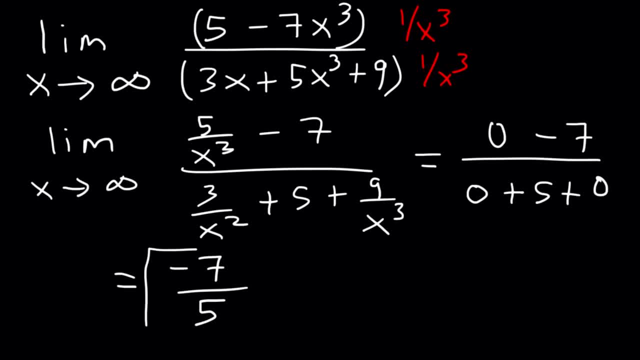 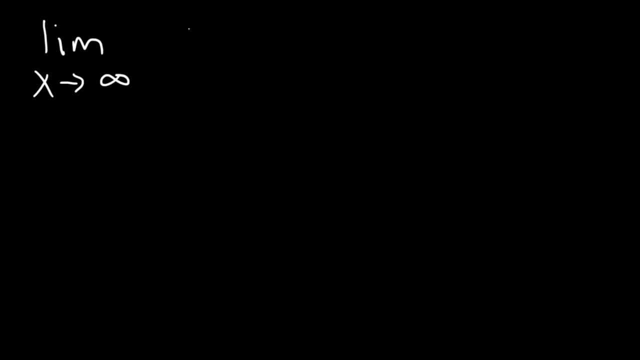 So in the end you get negative 7. Divided by 5.. What is the limit, as x approaches infinity, of the square root of 16x squared minus 8, divided by 2x minus 5?? Go ahead and try it. 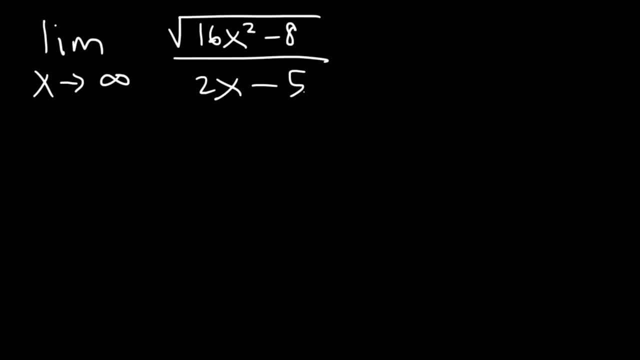 So when x is very large, only the most significant term will remain or will be important. 8 is insignificant and 5 is insignificant. So this expression: It becomes equal to the square root of 16x squared divided by 2x. 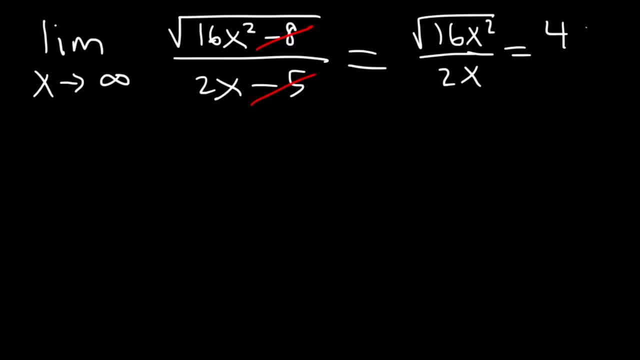 The square root of 16 is 4, and the square root of x squared is x, And 4x divided by 2x is 2.. So that's going to be the answer, But now let's confirm it with a step-by-step process. 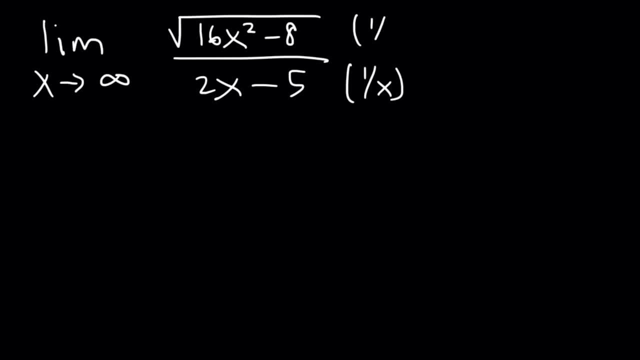 So we're going to multiply the top and the bottom by 1 over x. So on the bottom, 2x Times 1 over x is simply 2.. And then we're going to have 5 over x. 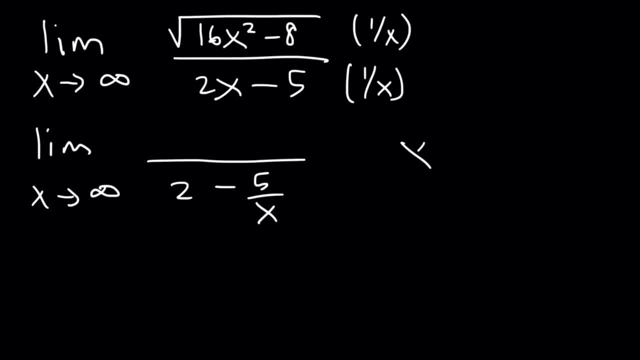 Now how do we put the 1 over x inside a square root? So let's say, if you have x root 2. And you want to move the x into the square root, You need to multiply the exponent by 2.. 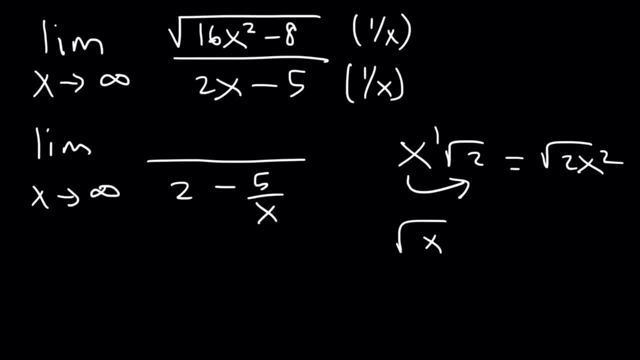 So it's going to turn into 2x squared, Because the square root of x squared is x. So if you want to move it back in you need to double the exponent, So to move in 1 over x into the radical. 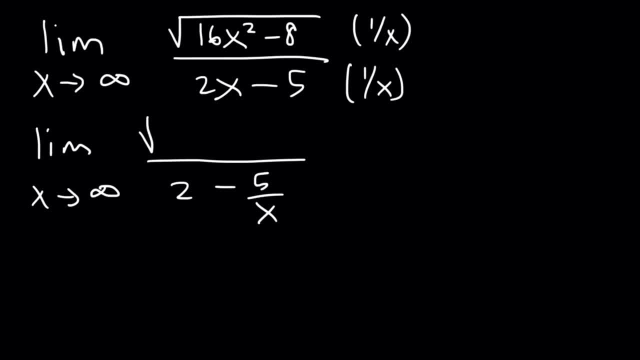 We need to multiply the inside by 1 over x squared, 16x squared times 1 over x squared. That's going to be just 16.. And then we're going to have 8 over x squared, Divided by 2 minus 5 over x. 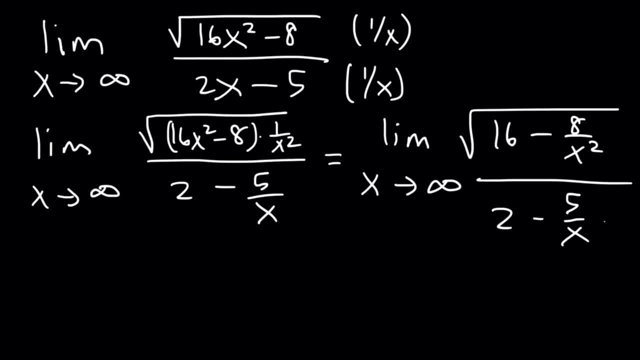 So now let's apply the limit as x approaches infinity To every term. It's not going to affect the 16. Because that's a constant 8 over x. squared, That's going to turn into 0.. And 5 over x. 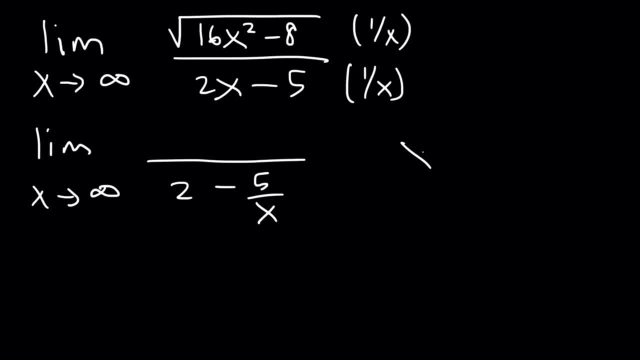 Now how do we put the 1 over x inside a square root? So let's say, if you have x root 2. And you want to move the x into the square root, You need to multiply the exponent by 2.. 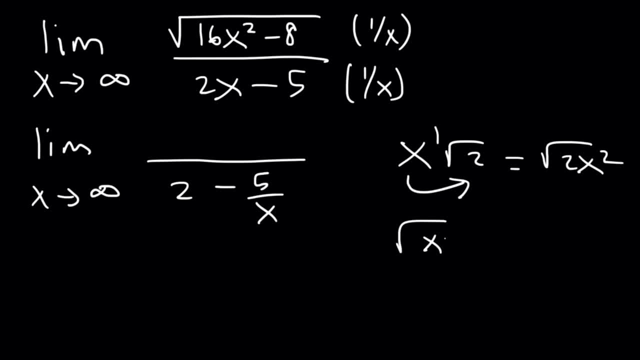 So it's going to turn into 2x squared, Because the square root of x squared is x. So if you want to move it back in you need to double the exponent, So to move in 1 over x into the radical. 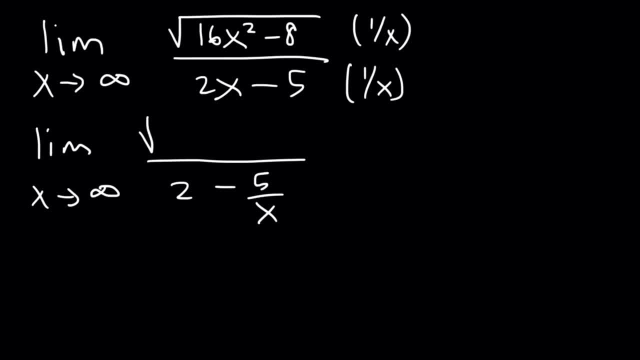 We'll need to multiply the inside by 1 over x squared, 16x squared times 1 over x squared. that's going to be just 16.. And then we're going to have 8 over x squared, divided by 2 minus 5 over x. 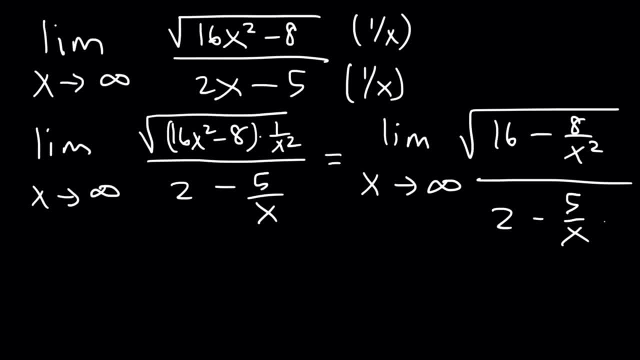 So now let's apply the limit as x approaches infinity to every term. It's not going to affect the 16, because that's a constant. 8 over x squared, that's going to turn into 0.. And 5 over x, that's going to be 0 as well. 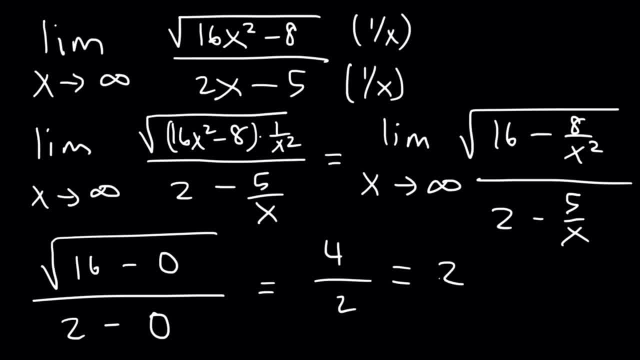 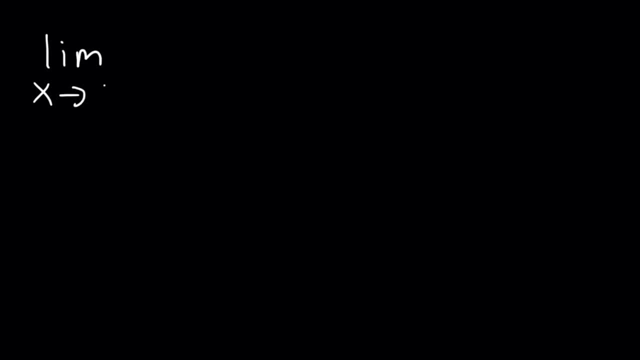 The square root of 16 is 4, so 4 divided by 2 is 2.. And that's going to be the answer. Now let's try this one. What is the limit, as x approaches infinity, Of the square root of 16?? 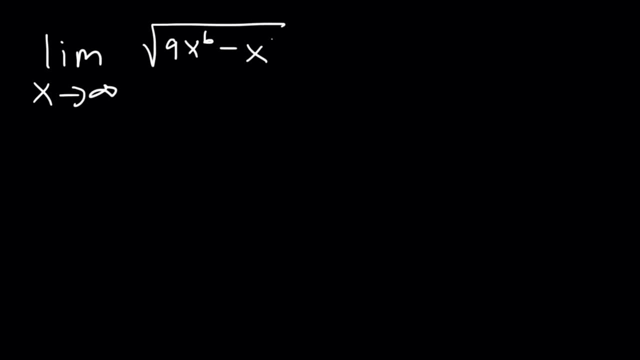 The square root of 9x to the 6th minus x, squared divided by 3x to the 3rd plus 1.. So we know that these terms are insignificant. So this becomes equal to the square root of 9x to the 6th over 3x cubed. 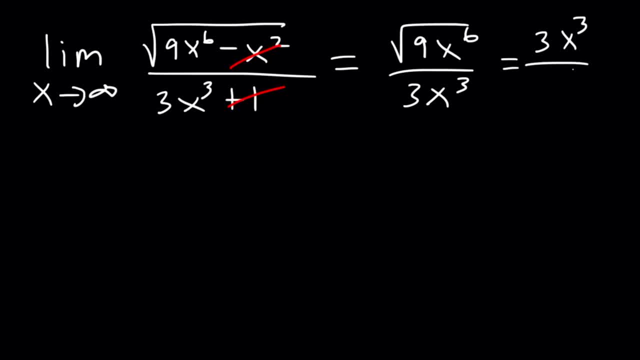 The square root of 9 is 3.. The square root of x to the 6th is 3x to the 3rd. So these two cancel. the final answer is 1.. Now to show you work, we can multiply the top and the bottom by 1 over x, cubed. 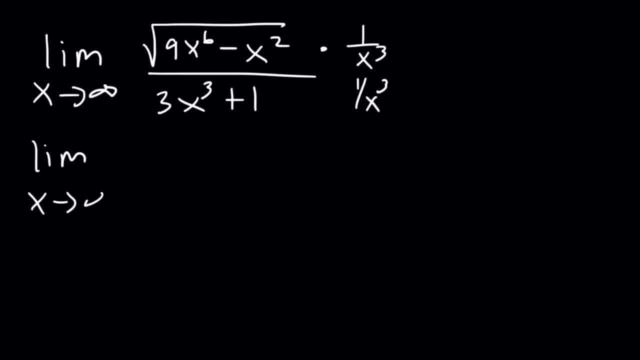 So this becomes the limit as x approaches infinity. And then on the inside we're going to have 1 over x cubed, actually x to the 6th. now The exponent will double once we move it to the inside. So 1 over x to the 6th times 9x to the 6th minus x squared. 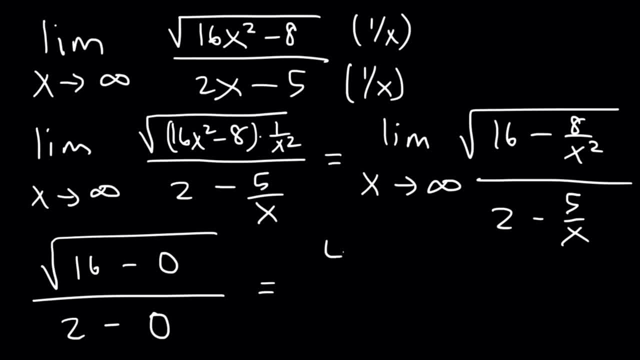 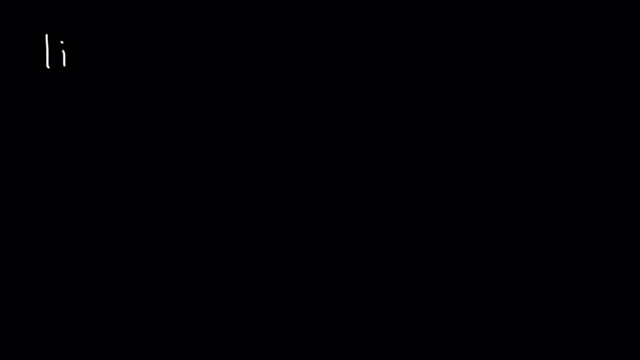 That's going to be 0 as well. The square root of 16 is 4.. So 4 divided by 2 is 2.. And that's going to be the answer. Now let's try this one. What is the limit as x approaches infinity? 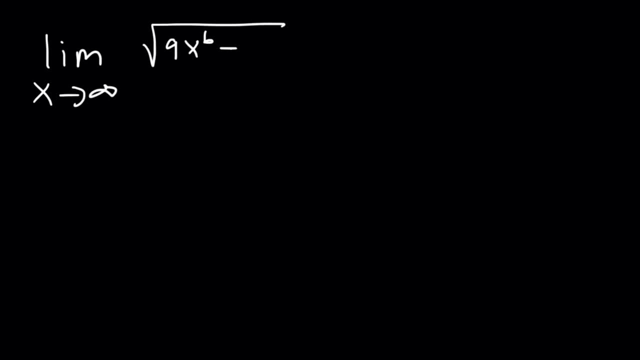 Of the square root of 9x to the 6. Minus x squared Divided by 3x to the 3rd plus 1.. So we know that these terms are insignificant. So this becomes equal to the square root of 9x to the 6 over 3x cubed. 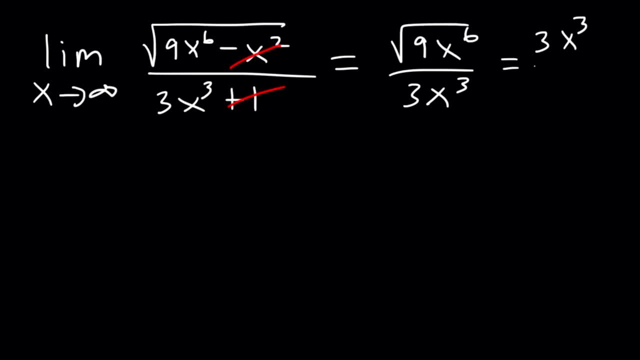 The square root of 9 is 3.. The square root of x to the 6 is 3x to the 3rd. So these two cancel. The final answer is 1.. Now to show you work, we can multiply the top and the bottom by 1 over x, cubed. 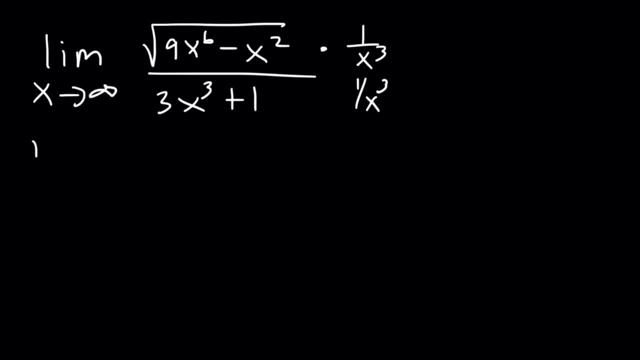 So this becomes the limit as x approaches infinity. And then on the inside we're going to have 1 over x, cubed, Actually x to the 6. now The exponent will double once we move it to the inside. 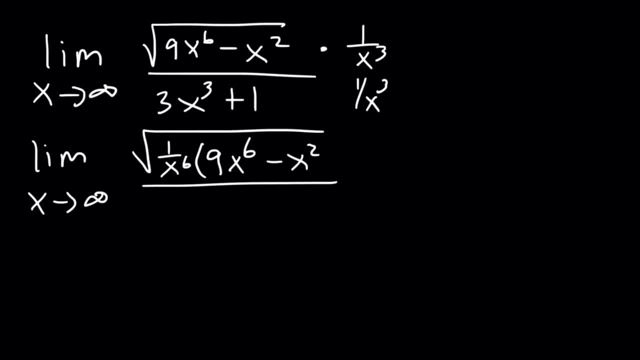 So 1 over x to the 6 times 9x to the 6 minus x squared, Divided by 3 plus 1 divided by x cubed. So now what we're going to do is rewrite this expression. 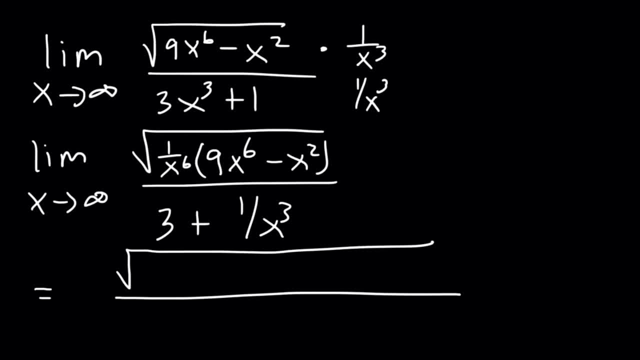 So this is going to be equal to the square root of 9 plus the limit as x approaches infinity, And that's going to be negative 1 over x to the 4th. That's negative x squared divided by x to the 6.. 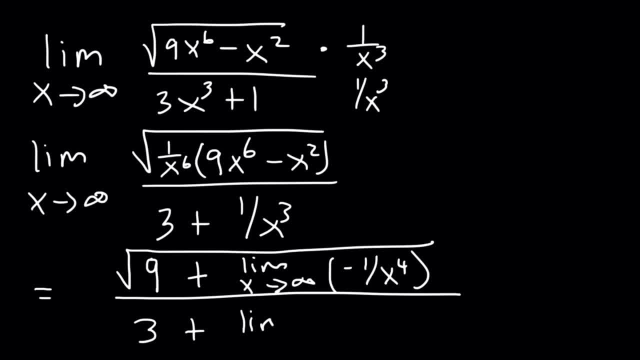 And then on the bottom we're going to have 3 plus the limit as x approaches infinity: 1 over x cubed. So this is going to become the square root of 9.. And the limit as x approaches infinity for 1 over x to the 4th, that's going to be 0.. 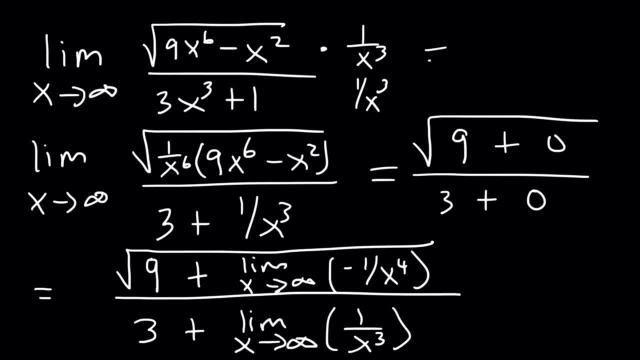 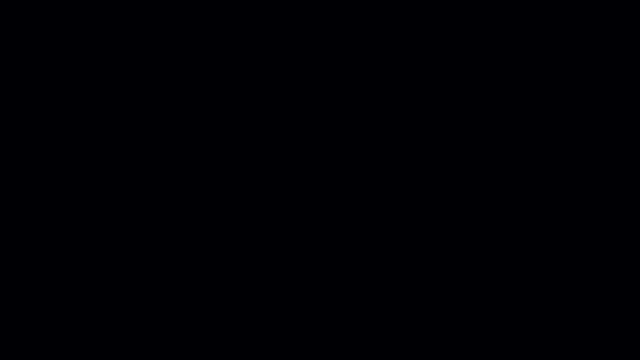 And for 1 over x cubed, that's going to be 0.. And then the square root of 9 is 3.. So 3 divided by 3 is 1.. What is the limit as x approaches infinity? 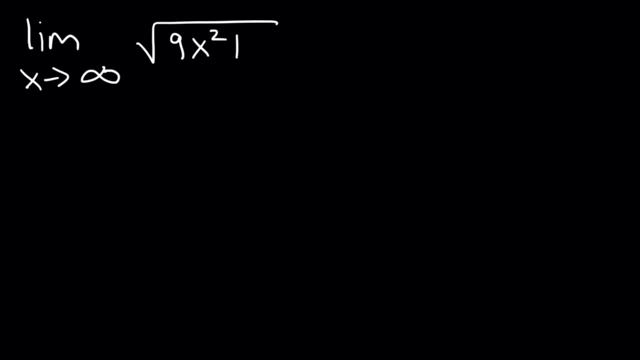 Of this function, the square root of 9x squared plus x minus 3x. What do we need to do here? What should we do? Well, if you're not sure what to do, use direct substitution. Plug in a very large number into the function. 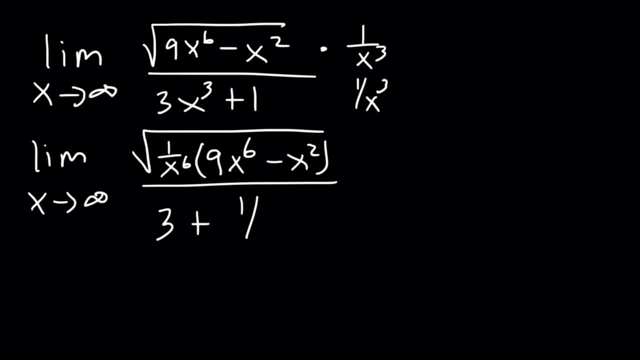 Divided by 3 plus 1 divided by x cubed. So now what we're going to do is rewrite this expression. So this is going to be equal to the square root of 9 plus the limit as x approaches infinity, And that's going to be negative 1 over x to the 4th. 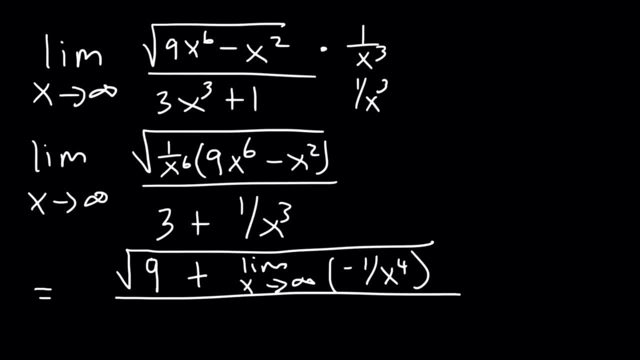 That's negative x squared divided by x to the 6th, And then on the bottom we're going to have 3 plus the limit as x Approaches infinity, 1 over x cubed. So this is going to become the square root of 9.. 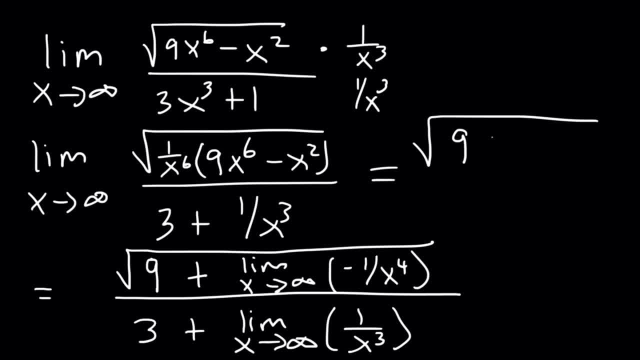 And the limit as x approaches infinity. for 1 over x to the 4th, that's going to be 0.. And for 1 over x- cubed, that's going to be 0.. And then the square root of 9 is 3.. 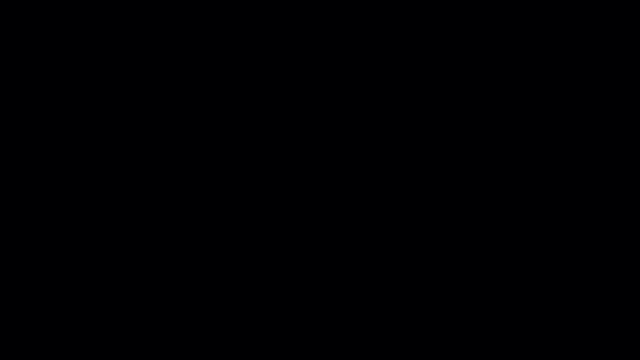 So 3 divided by 3 is 1.. What is the limit, as x Approaches infinity, of this function, The square root of 9x squared plus x, minus 3x. What do we need to do here? What should we do? 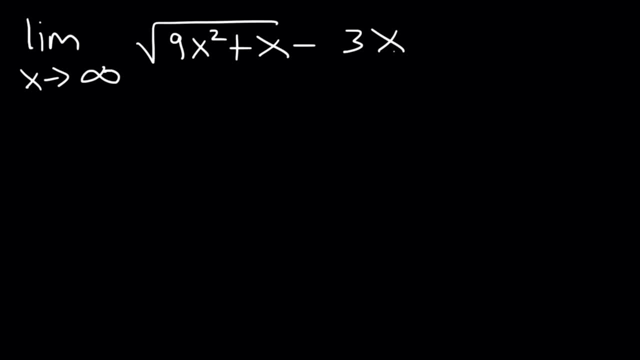 Well, if you're not sure what to do, use direct substitution. Plug in a very large number into the function, So let's use 1,000.. So 9 times 1,000 squared plus 1,000.. Minus 3 times 1,000.. 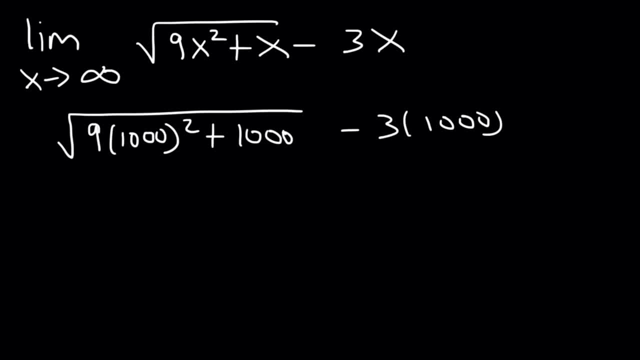 Now, if you type this whole thing in, you should get 0.1666620373.. Which is basically 1 over 6.. Which is 0.16 repeated. So 1 over 6 is the exact answer. But now, what techniques can we use to actually get that answer? 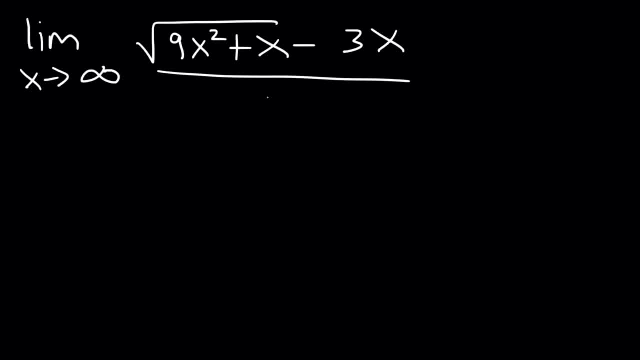 The first thing you should do is write this as a fraction, Put it over 1.. And then multiply the top and the bottom by the conjugate. That is 9x squared plus x plus 3x. So when we FOIL the binomials on top, the two middle terms will cancel. 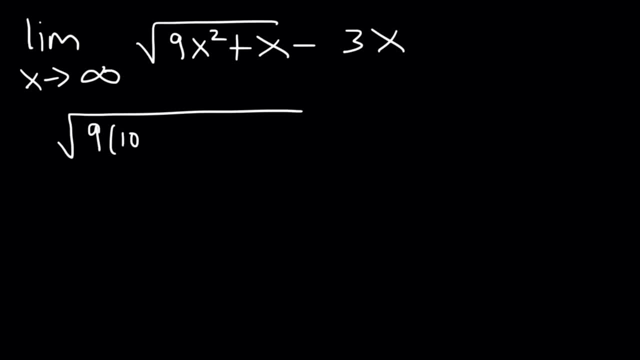 So let's use 1,000.. So 9 times 1,000 squared plus 1,000, minus 3 times 1,000.. Now if you type this whole thing in, you should get 0.1666620373.. 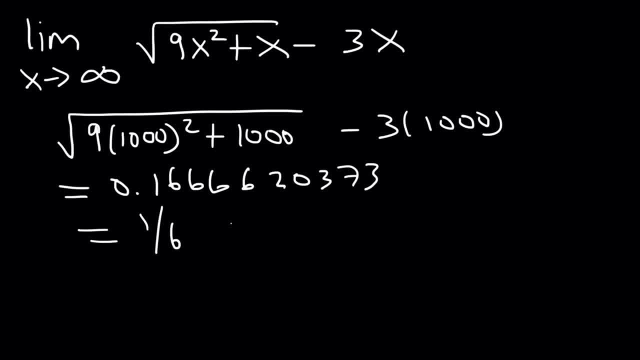 Which is basically 1 over 6.. Which is 0.16 repeated. So 1 over 6 is the exact answer. But now what techniques can we use to actually get that answer? The first thing you should do is write this as a fraction: 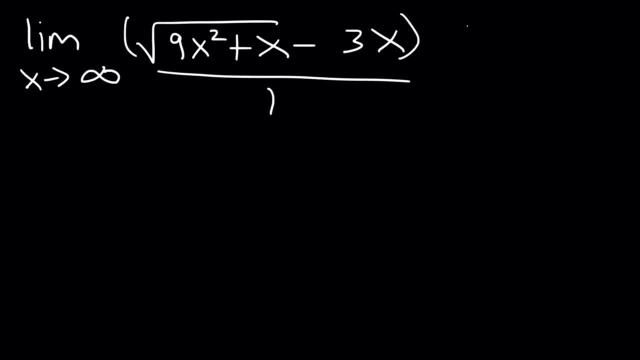 Put it over 1. And then multiply the top and the bottom by the conjugate, That is 9x squared plus x plus 3x. So when we FOIL the binomials on top, the two middle terms will cancel. 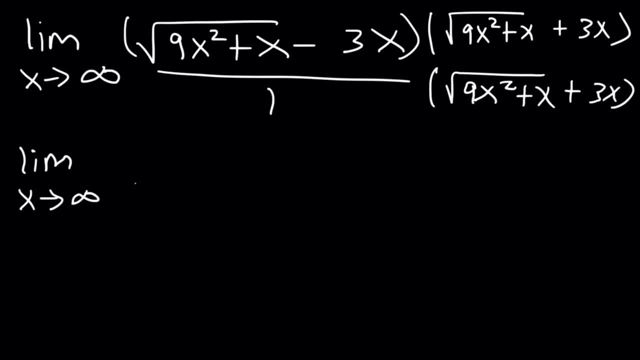 So what we're going to have is the limit, as x approaches infinity, of 9x squared plus x, The square roots cancel And then 3x times 3x is 9x squared. But that's going to be. 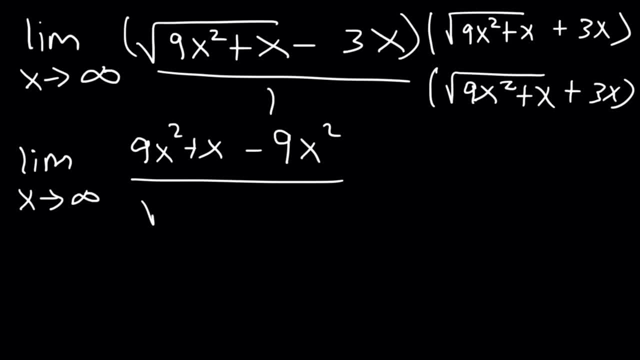 Negative: 9x squared. Divided by what we have here, These two add up to 9.. So we can get rid of it. So, based on what remains, we're going to multiply the top and the bottom by 1 over x. 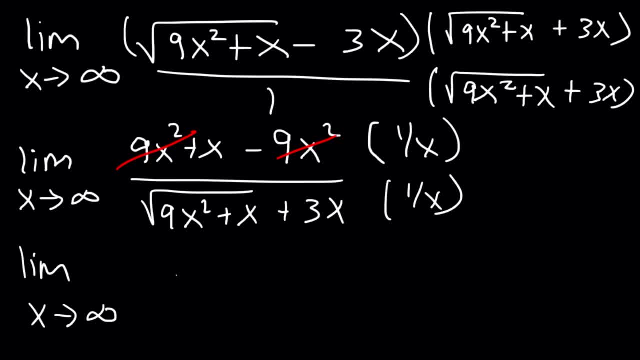 So this is going to be the limit as x approaches infinity. x times 1 over x is 1.. Now, inside the radical, we need to multiply it by 1 over x squared. 9x squared times 1 over x squared is going to be 9.. 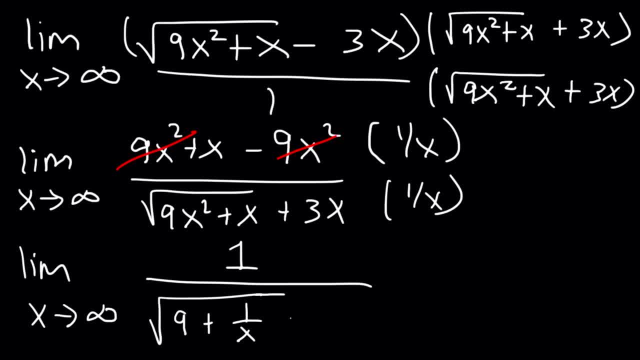 x times 1 over x, squared is going to be 1 over x, And 3x times 1 over x is just 3.. So now all we do, All we need to do, excuse me, is apply the limit to 1 over x. 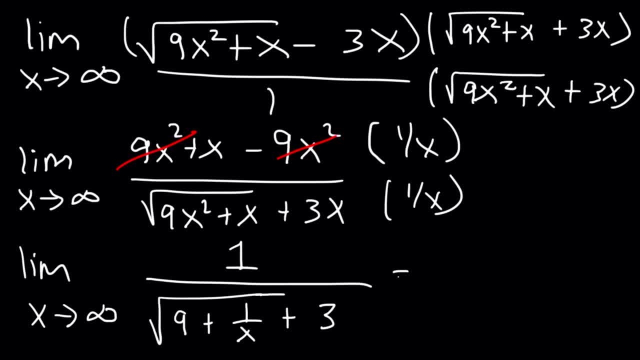 The limit, as x approaches infinity, of 1 over x is 0.. So this is going to be 1 divided by the square root of 9 plus 0 plus 3.. Okay, We know, the square root of 9 is 3.. 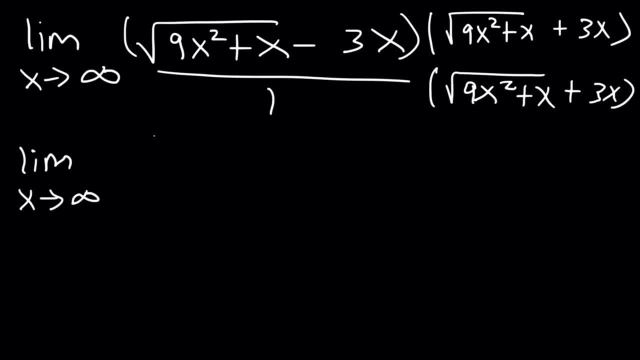 So what we're going to have is the limit, as x approaches infinity, of 9x squared plus x, The square roots cancel And then 3x times 3x is 9x squared, But that's going to be negative 9x squared. 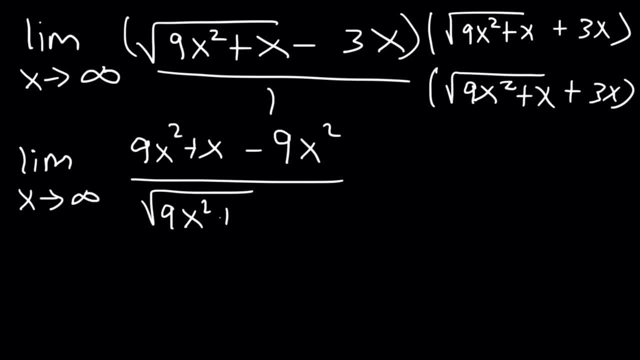 Divided by what we have here, These two add up to 9.. So we can get rid of it. So, based on what remains, we're going to multiply the top and the bottom by 1 over x. So this is going to be the limit as x approaches infinity. 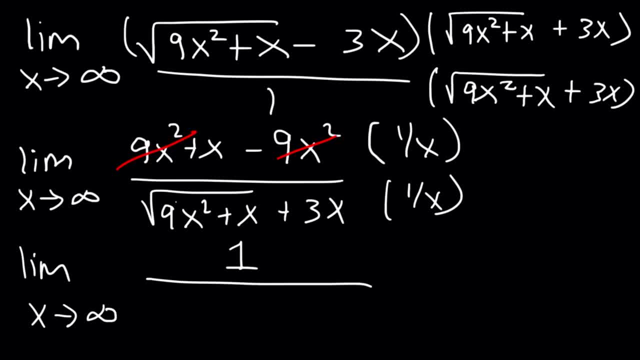 x times 1 over x is 1.. Now inside the radical, we need to multiply it by 1 over x squared. 9x squared times 1 over x squared is going to be 9.. x times 1 over x squared is going to be 1 over x. 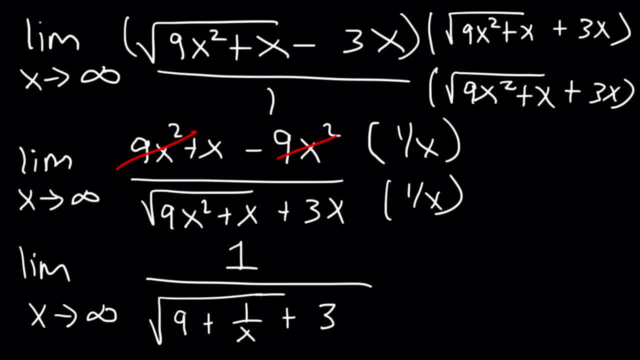 And 3x times 1 over x is just 3.. So now all we need to do is apply the limit to 1 over x. The limit, as x approaches infinity, of 1 over x is 0.. So this is going to be 1 divided by the square root of 9 plus 0.. 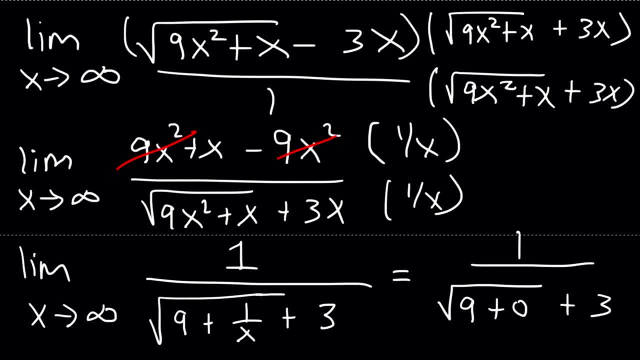 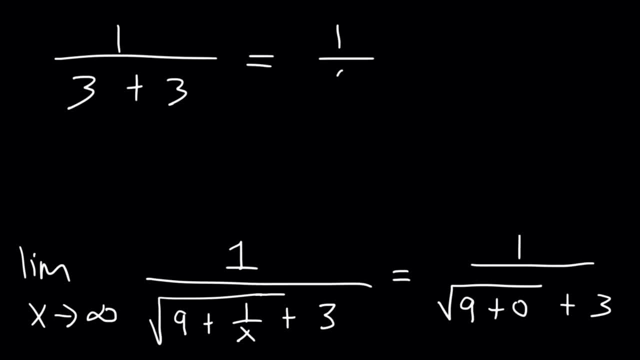 And we know the square root of 9 is 3. And 3 plus 3 is 6.. So the final answer, as you mentioned before, is 1 over 6.. What is the limit as x approaches infinity, of the function arctangent of x? 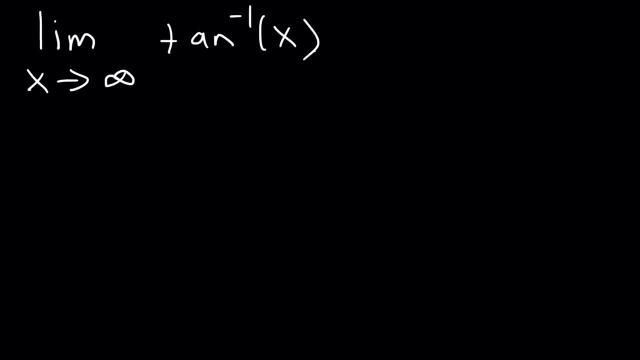 So what is the arctan of infinity? Well, let's plug in points. So first put your calculator in degree mode. So if we plug in arctan of 100, this is 89.4.. Now if we plug in arctan of 1,000,, 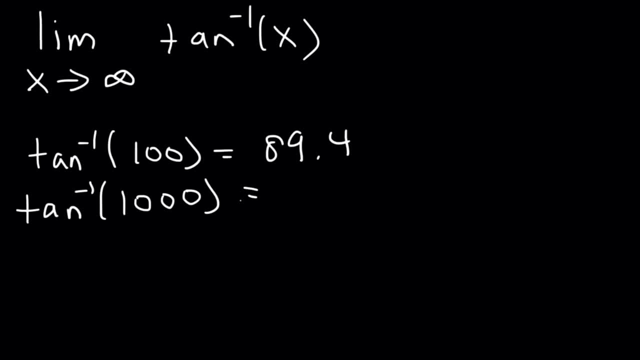 this is 89.94.. Notice that it gets closer and closer to 90.. So this is 89.94.. Notice that it gets closer and closer to 90.. This is equal to 90 degrees or in radians pi over 2.. 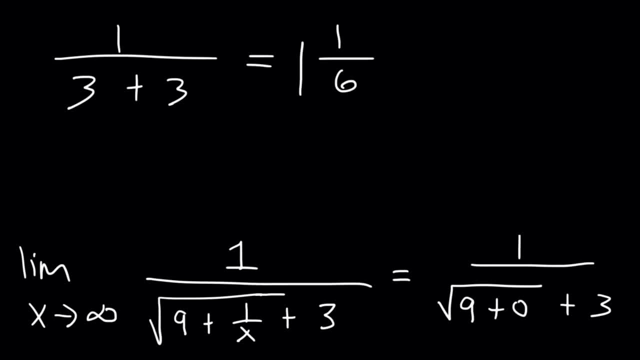 And 3 plus 3 is 6.. So the final answer, as you mentioned before, is 1 over 6.. What is the limit, as x approaches infinity, of the function arctangent of x. So what is the arctan of infinity? 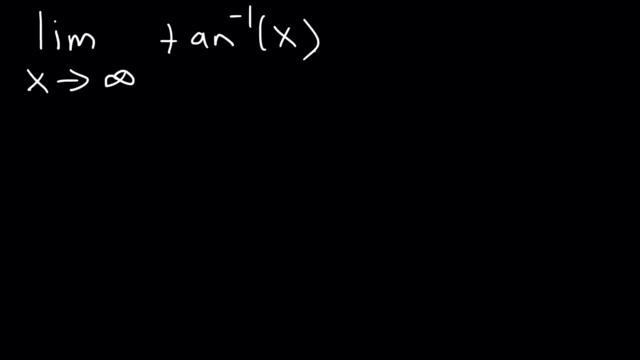 Well, let's plug in points. So first put your calculator in degree mode. So if we plug in arctan of 100, this is 89.4.. Now if we plug in arctan of 1,000, this is 89.94.. 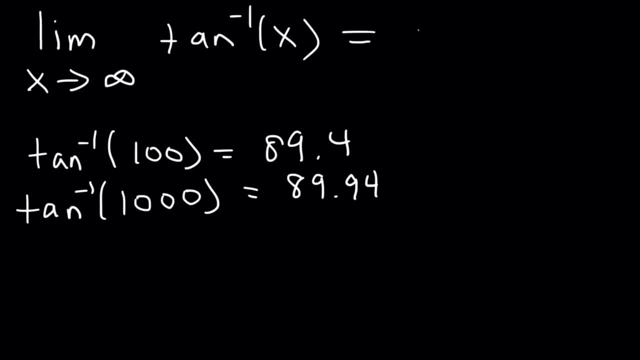 Notice that it gets closer and closer to 90. So this is equal to 90 degrees or, in radians, pi over 2.. Now, if we recall the limit as tangent or as x approaches pi over 2 from the left side of tangent x, 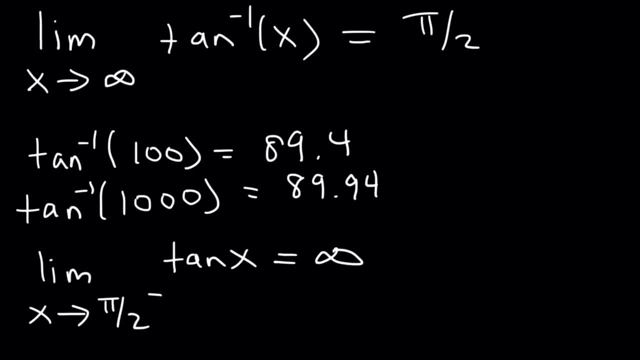 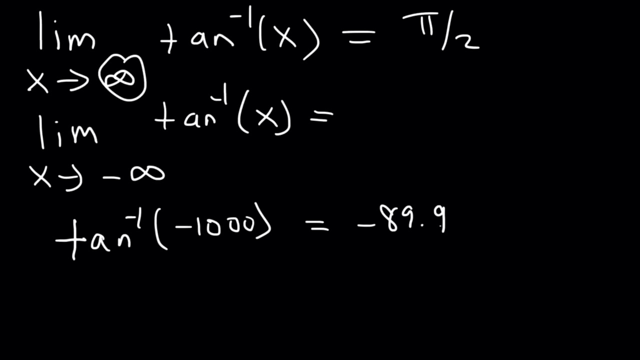 that's equal to infinity. So when dealing with inverse tangent you need to switch these two values. Now what is the limit as x approaches negative infinity? So if we plug in arctan of negative 1,000, while it's in degree mode, this is going to be negative 89.9.. 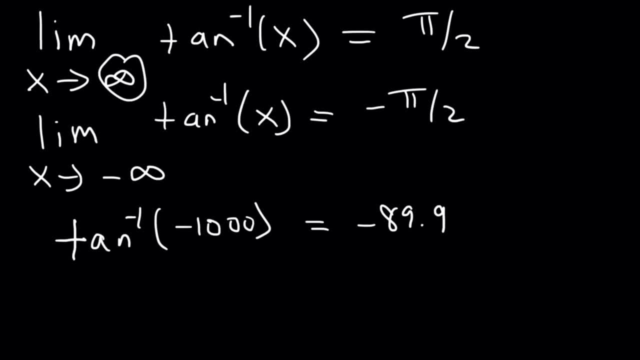 So this is negative pi over 2, or basically negative 90.. Tangent is negative in quadrants 2 and 4, but arctan only exists in quadrants 1 and 4.. So that's why we got the answer that's in quadrant 4.. 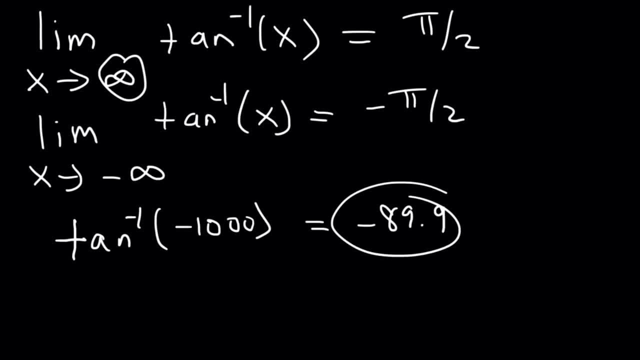 Negative 89.9, which gets it very close to negative 90, or negative pi over 2.. So make sure you know these values. Now there's one more that we need to go over: What is the limit, as x approaches infinity, of e to the negative x? 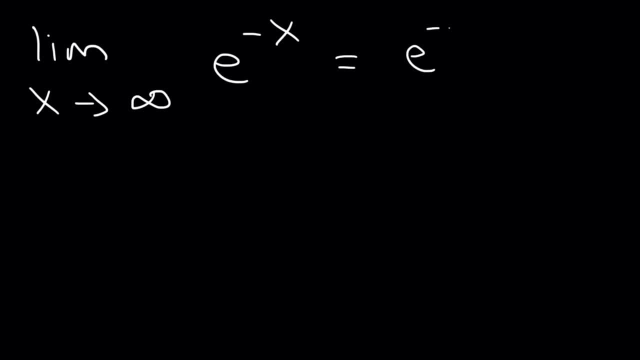 What is the answer? So if we plug in infinity, this is going to be e to the negative infinity, which is 1 over e to the infinity. e to the infinity is infinity and 1 divided by infinity is 0..